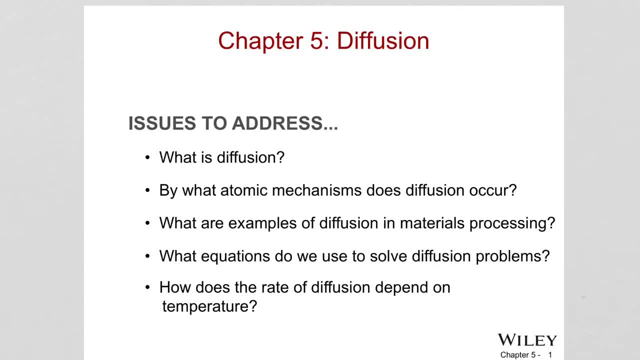 So today's topic is diffusion. Many processes and reactions in materials involves the diffusion of atoms, like heat treatments, corrosion, many significant processes that are taking place in a material system. It always includes diffusion. So it is very important to understand diffusion, the flow of atoms, and what are the factors that are affecting. 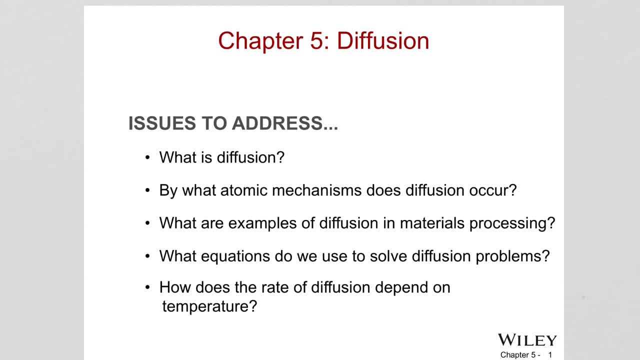 And one example I just remember. for example, oxidation, phase changes, phase transformations, going from one phase to another, all these type of processes that are taking place in a material system. they all include atomic motion. right, That is what we call diffusion, net flow of atoms due to a concentration gradient. So therefore, we're going to cover diffusion in this chapter. 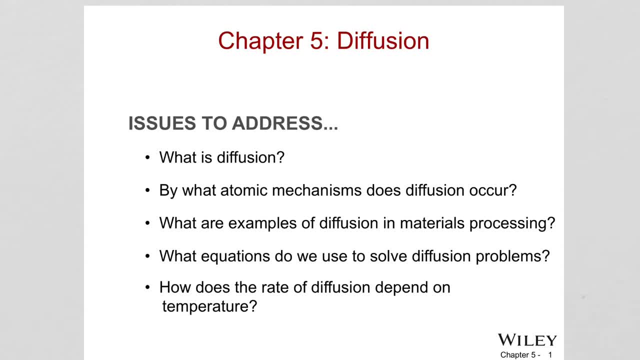 So these are the questions we're going to look: What is diffusion And what type of diffusions there are And what are examples of diffusion? So there are a lot of diffusions in material processing And the mathematical equations we use to describe the diffusion, the atomic motion. 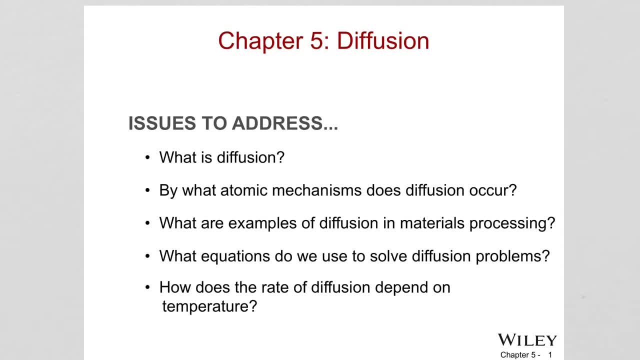 And of course, the temperature is very important in determining the rate of diffusion, because diffusion is what we call thermally activated process. As the temperature increases, diffusion also increases. That is the reason why, at high temperature, materials are more susceptible to corrosion, because corrosion is a process where atomic motion is very important, and when we increase the temperature, this atomic motion, atom movements, the rate of them is increasing. therefore corrosion is increasing. 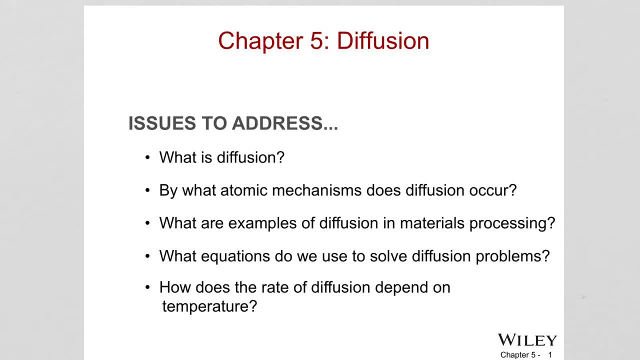 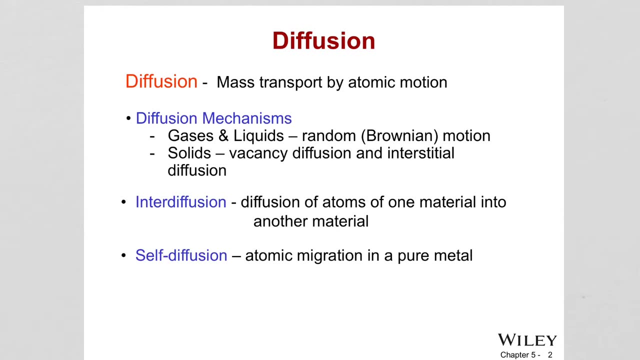 So how are we going to see how the rate of diffusion depends on the temperature? So these are the questions we're going to look. Okay, as I said, diffusion is defined by mass transport, by atomic motion, So the mechanism of diffusion is in gases and liquids. It's just a random motion. 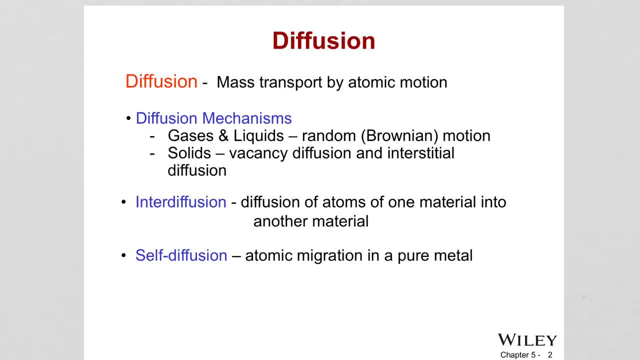 And in solids there is vacancy diffusion- We're going to learn- And interstitial diffusion. So interdiffusion is diffusion of atoms of one material into another- So we're going to see an example- And self-diffusion is atomic migration in a pure metal. 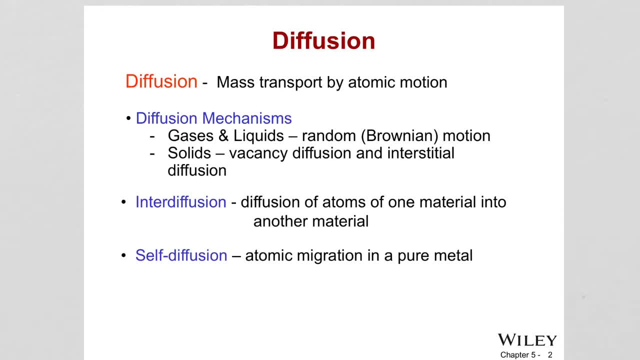 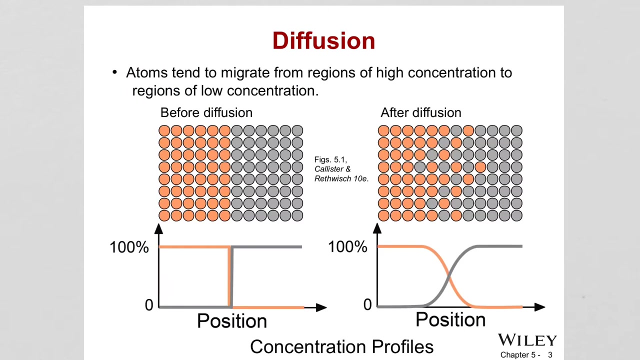 So it is basically all atoms exchanging positions are of the same. So when this is self-diffusion, But the process of by which atoms of one metal diffuse into another, that is called interdiffusion. Okay, let's see examples. So one thing we need to understand is there has to be a concentration gradient or concentration difference as a driving force for atoms to move, to go from one place to another. basically, 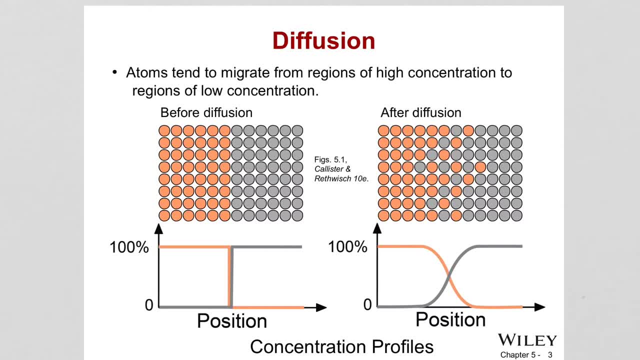 Okay. and the tendency for this? of course atoms. they tend to migrate from regions of high concentration to low concentration. So let's say we have a diffusion cup Couple, the copper and nickel metals bars are joined together. Let's say these orange atoms are copper and the gray ones representing nickel. 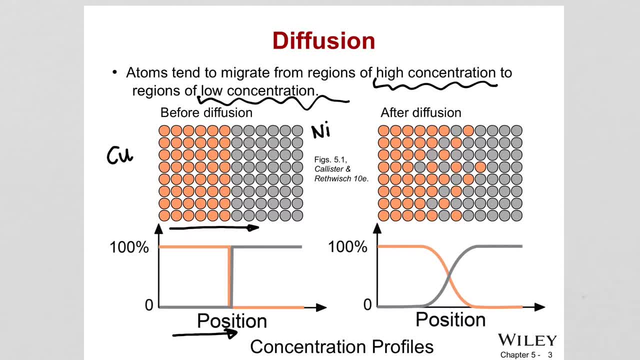 And they are joined, And then this couple is heated to an elevated temperature. but it should not be heated, It should be below the melting point. Okay, below the melting point, their melting points, and then heated to an elevated temperature and keep kept that temperature for a certain period of time. 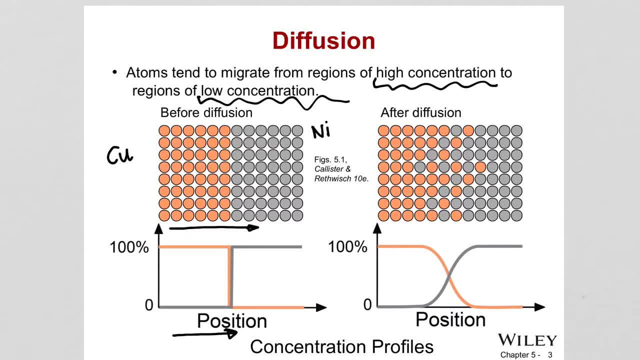 So, before we do that, if we look at the, if we look- actually, let's erase this- How, with position, the concentration of copper and nickel atoms are changing. So remember, orange is the copper right. So, and I am looking at the graph with position, 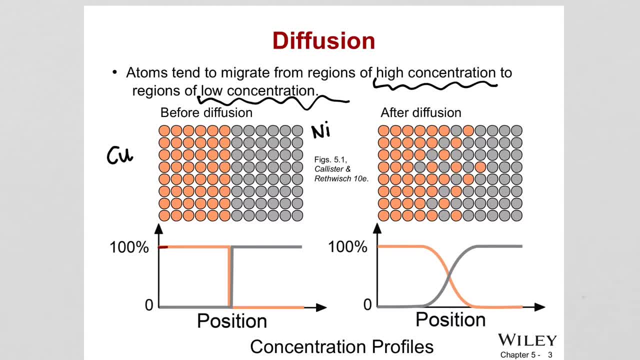 So initially here, when I move along the material edge, So it is 100% copper, copper, copper, copper. But when I come to the interface, suddenly a drop to 0% of copper, because it's all nickel and copper concentration is zero here. 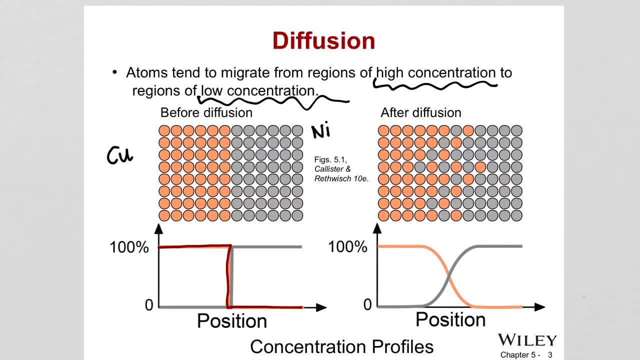 But when you look at the nickel along the position, as a function of position, it is 0, 0, 0% nickel, And when I reach the interface, suddenly there is we go to 100% copper. So this is before. we are actually just attaching, just putting these materials together, but not doing any heat treatment. 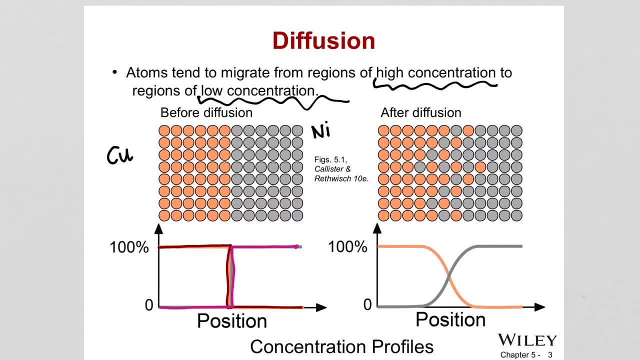 But after we increase the temperature and kept the material, this couple, at that temperature for a certain period of time, And then after that we cool it down back to the room temperature, And then let's say we are doing chemical analysis And we want to look at 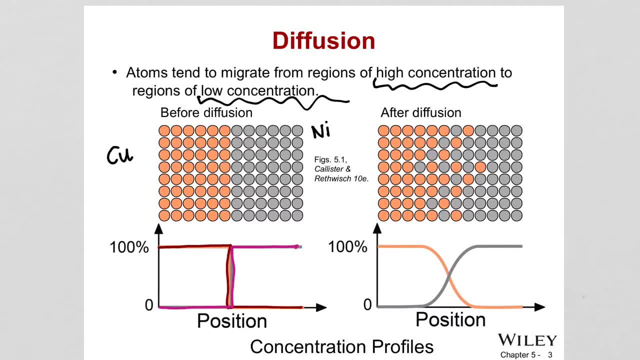 We want to look at how the interface looks like now. Okay, So after diffusion. of course, with the heat, some diffusion takes place, right? Atoms move towards each other. They're going to move from where they are at high concentration to where they are at low concentrations. 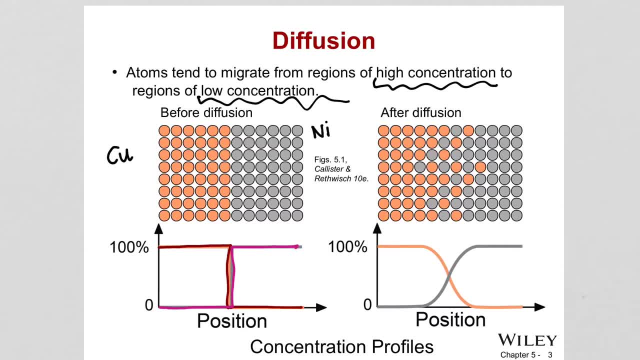 So copper is going to move towards nickel because inside the nickel there is low concentration of copper. Of course the nickel is going to move towards nickel. It's going to move towards copper because inside copper it's at low concentration, right? 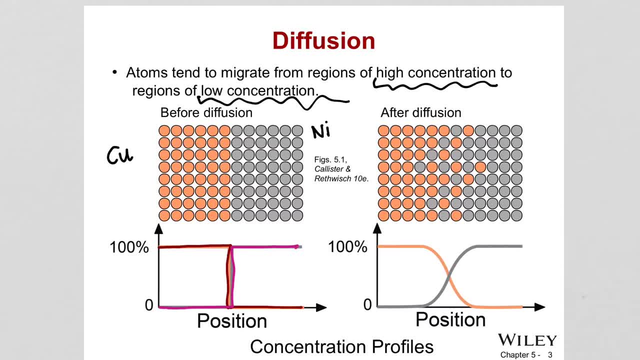 So they are moving towards each other And therefore, if we look at the same diagram for the, how the concentration changes as a function of position after the diffusion takes place, We can see that if we look at- let's choose the colors First, let's look at the copper. 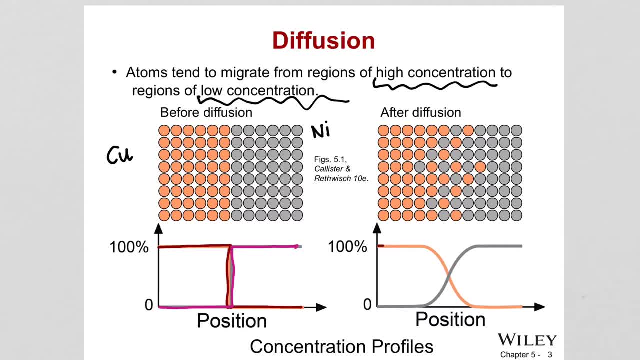 Again, far away from the interface, we still have 100% copper. But now, when we approach towards the interface, the concentration decreases, But not an abrupt decrease, right Slowly decreases and then reaches 0%. And the same is for the copper nickel now. 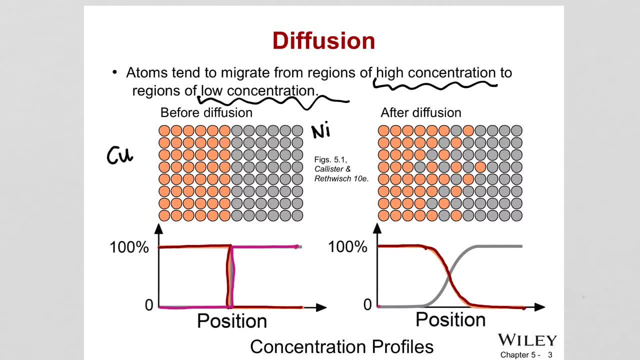 Right. So as we reach the interface, it is quickly increasing the nickel concentration And then it is reaching 100% when we are far away. So this is what they observe right And when they did this experiment. So these are concentration profiles that are showing us that when we actually form couples like that, 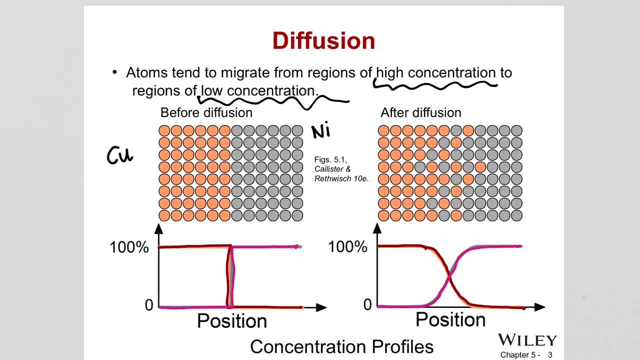 And give them some energy, like heat, The atoms will have enough energy and enough driving force because there is concentration difference And they will move towards each other, diffuse to each other. Okay, So in this case, this is an example of interdiffusion. 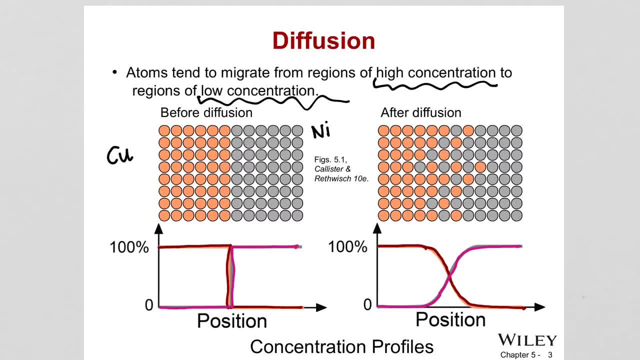 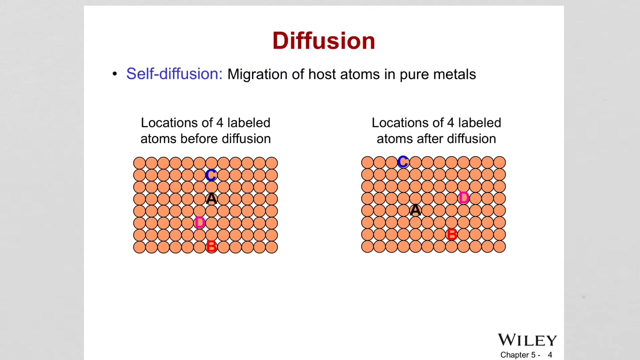 Right, Because the copper have migrated into nickel And nickel have migrated into copper here, Right? So let's write it down. Okay, This is interdiffusion example. Okay, So we said the self-diffusion was migration of host atoms in pure metals. 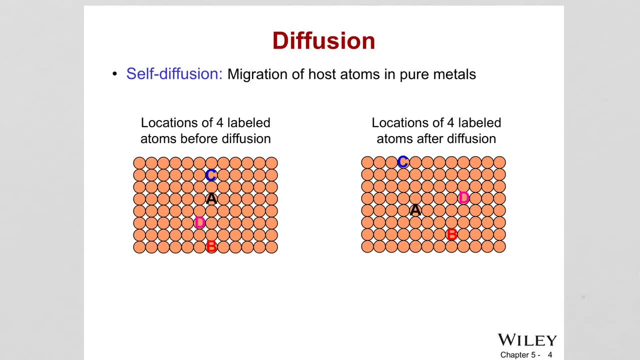 So to be able to understand that of course we are looking at a pure metal Right. So all atoms, they are the same. So we might be thinking: How come these atoms are going to move? And actually that is always happening in a material. 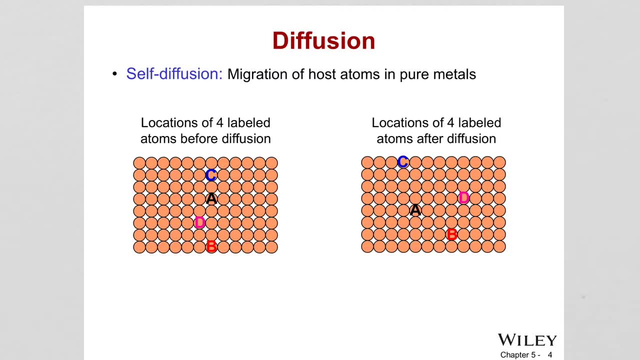 So the atom doesn't stay in its position? Okay, It moves around the material. That's what we call self-diffusion in a pure material. So to be able to, of course understand that, since all atoms are the same, We have labeled the atoms. let's say A, B, C, D, A atom, B atom and D atom. 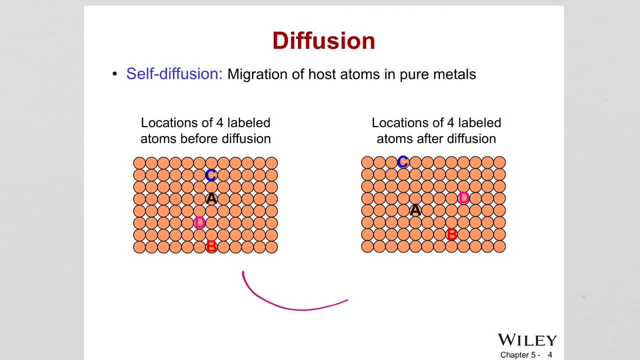 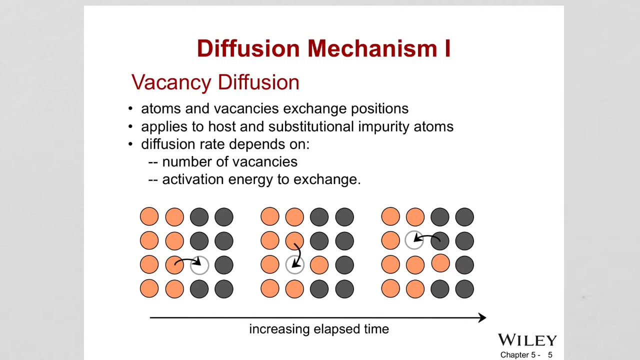 And when diffusion takes place, actually all those atoms are now in different places. Of course the material will look like the same to you, But those atoms actually moved along inside the material. So let's look at different diffusion mechanisms. The first one is vacancy diffusion. 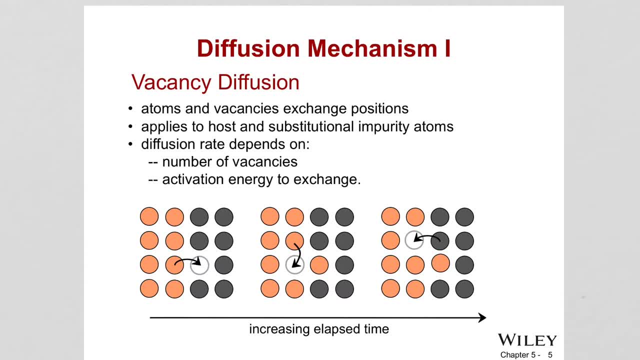 So, as the name implies, this involves the interchange of an atom from its normal lattice position to an adjacent vacant site or vacancy, And this is also shown schematically here. Okay, So For Vacancy diffusion to take place, there has to be vacancy sites in the structure. 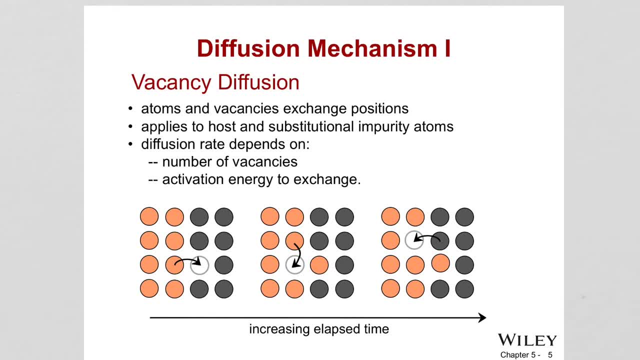 And we learned the equilibrium number of vacancies that are in the material and how it is affected with the temperature Right. So there is always vacancies present, But when we increase the temperature, The concentration of vacancies increase. So this also affects the vacancy diffusion. 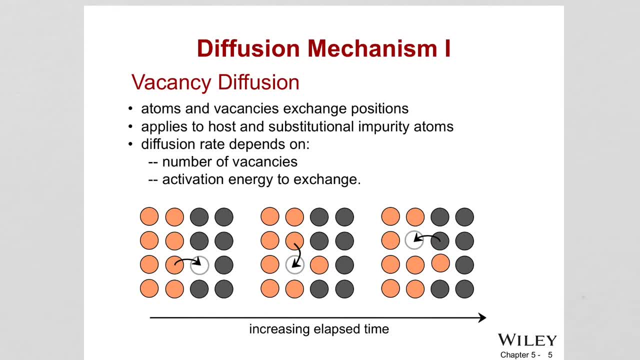 Because for vacancy diffusion to take place there has to be vacancies in the structure And of course the atom needs to have a certain energy to be able to move from its original spot to the vacancy site. So Atomic motion and the vacancy site. 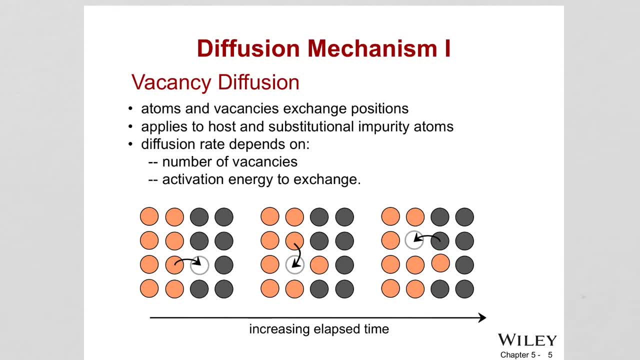 So atomic motion and the vacancy motion are happening in opposite directions, of course, Because, as we see in this- let's say, this is the same copper and nickel couple- The copper is diffusing into the vacancy site here. Right, Let me draw it again. 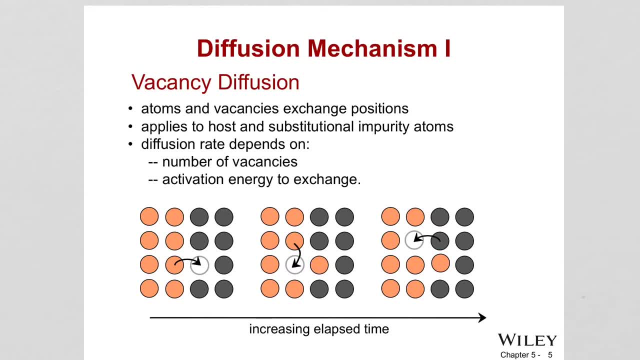 So copper is from here Right Going to the vacancy site here. So copper motion is going this direction. Of course, when this happened, vacancy moves towards the copper Okay. So vacancy comes here, The copper atom goes there. Both self diffusion and inter diffusion occur by this mechanism. 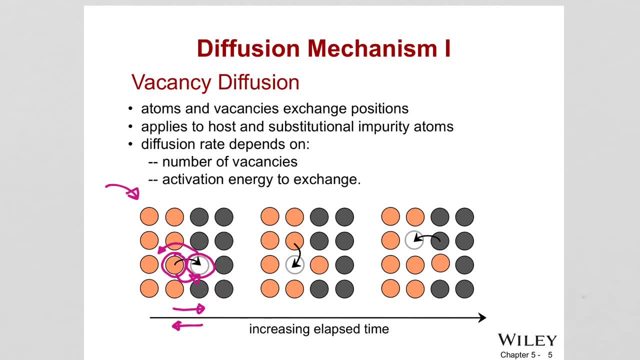 And in self diffusion, of course, The pure metal, pure atoms in the pure metal, will exchange positions with the vacancies. And the example for the inter diffusion is here: The copper and nickel copper Right, Like the one we've seen Right. 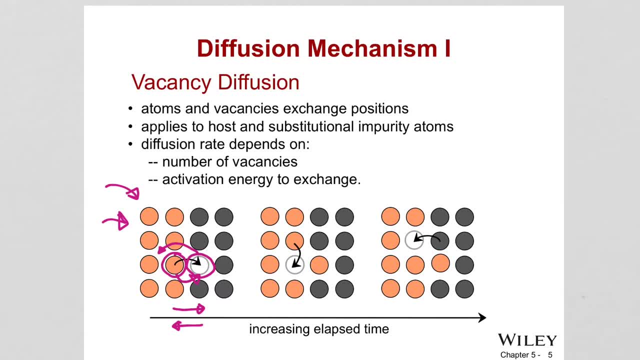 So of course, the diffusion rate will depend on, as we said, the number of vacancies And the activation energy to exchange Position with the vacancy. As we are seeing in the image now, the vacancy moved here in the structure Right. 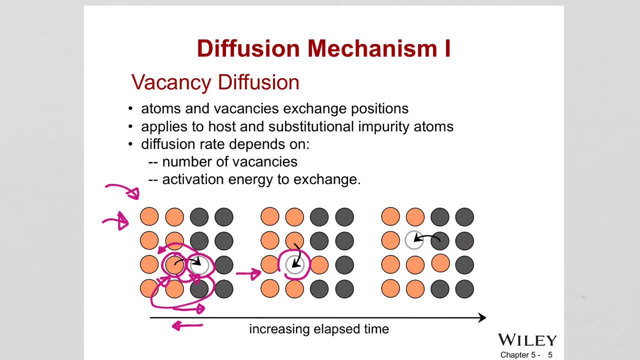 From here to here it moved. So when we go to the next image of the same material, now vacancy is right here, And now another atom will move towards the vacancy site, So this will come here And this place will be vacancy. 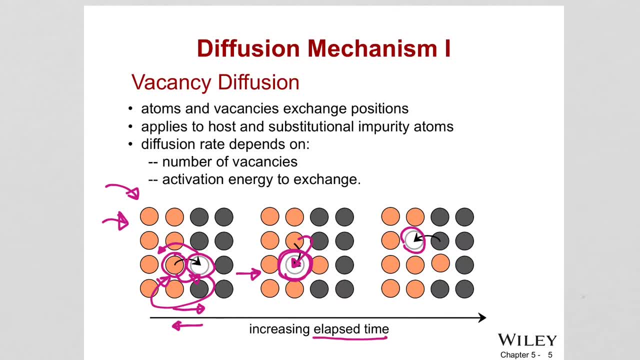 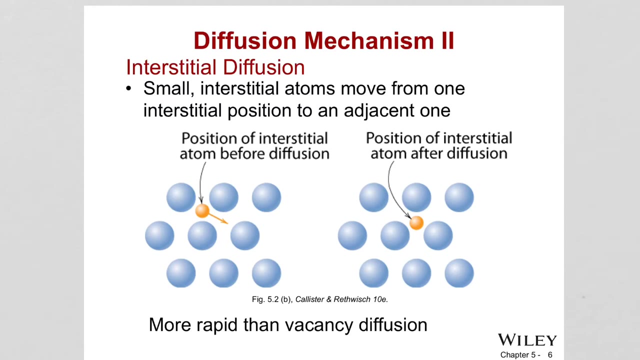 So this is, with time, how the material, how the vacancy is moving, or how the atoms are moving along inside the material. Okay, So another diffusion mechanism is interstitial diffusion. This involves atoms that migrate from an interstitial position to a neighboring one that is empty. 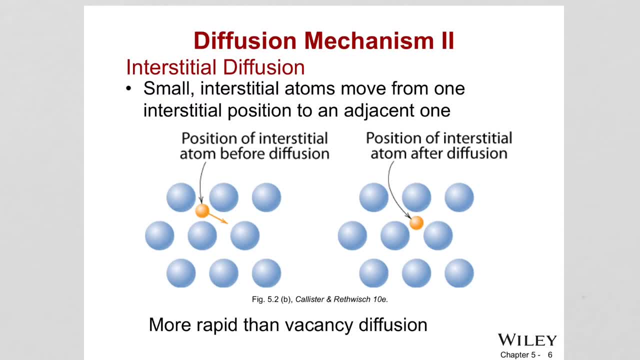 This mechanism is especially important for inter diffusion of impurities, Impurities like hydrogen, carbon nitrogen and oxygen. It is easy to understand Right. Basically, the atoms that are in interstitial positions move from one interstitial position to another. 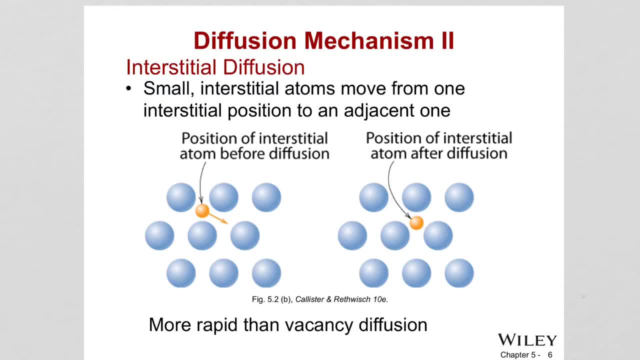 So this is more rapid than vacancy diffusion. And think about why this can be. One reason is interstitial atoms are smaller, So they can easily move. Okay, They are more mobile And also the probability of having another empty interstitial site is much higher compared. 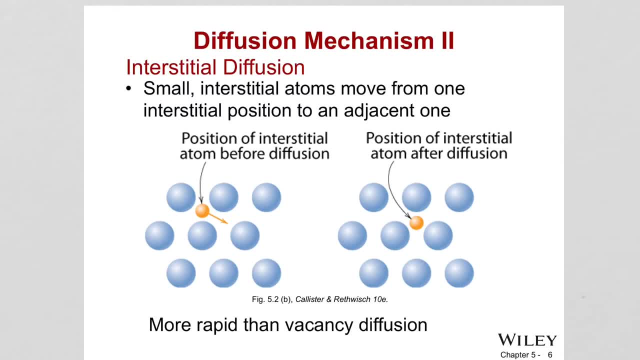 to having a vacancy position next to the atom. So therefore this is like a probability also, Right? So the probability of having a vacancy next to the atom is much less than the probability of having an interstitial site, The probability of having an empty interstitial site next to another interstitial site. 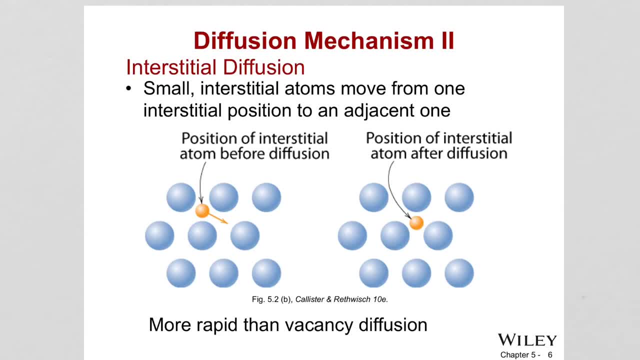 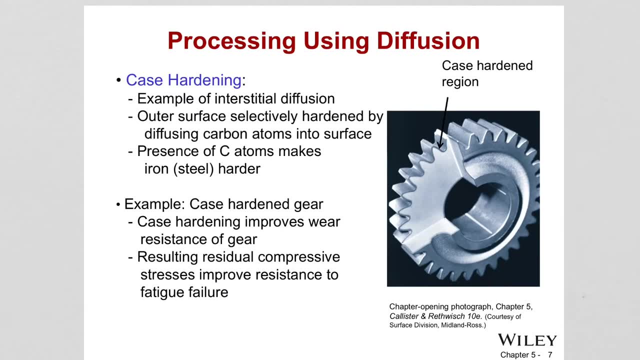 Therefore, interstitial diffusion is faster than vacancy diffusion. Okay, So we are given an example. There were a process, a material processing technique- Okay, Where the diffusion is important. This material processing technique is called case hardening And this is done to enhance the surface properties of a material. 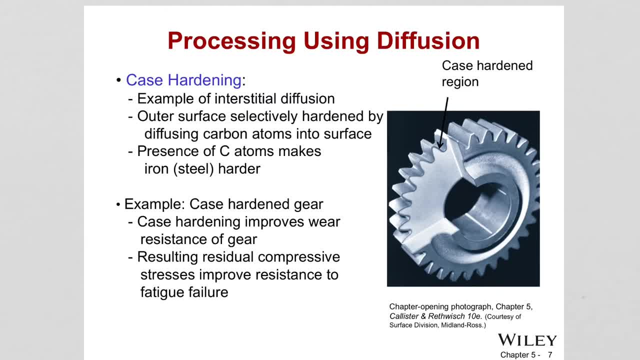 So how it is done. Basically, carbon atoms are diffused. Carbon atoms are diffused into the iron on the surfaces. Let's say we have a gear like shown in the image And outside this region you can see difference in color also. 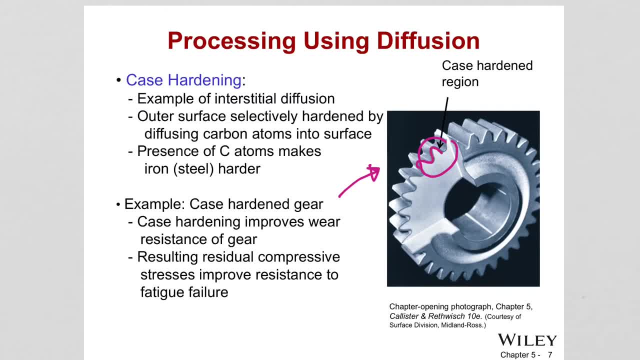 The surface that is hardened by the diffusion of carbon atoms into the surface. So why do we do that? Because it enhances the properties like wear resistance of the gear And improve properties like resistance to fatigue failure, Which we gonna see later in chapter 6 when we look at mechanical properties. 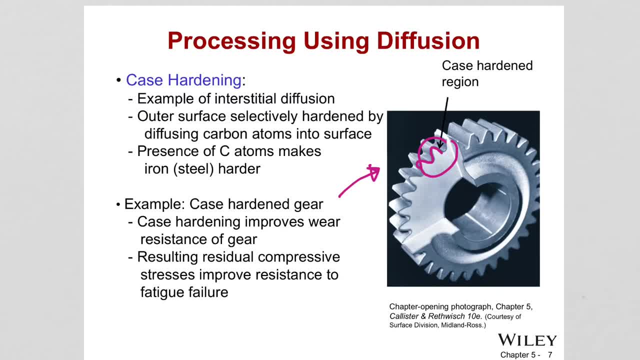 What is fatigue, failure, etc. But this is just a surface treatment of materials, Where we use diffusion of carbon to enhance the surface characteristics of certain materials And an example of how diffusion is important to understand How diffusion is affected with certain parameters like temperature, temperature, concentration, gradients, etc. 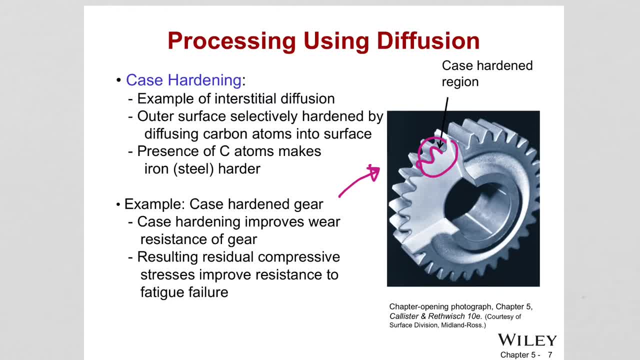 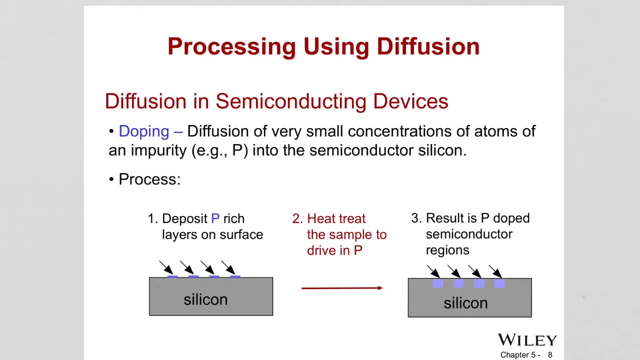 So when we look at the mathematical equations We gonna understand what parameters are affecting the diffusion and diffusion rate. Another example where the diffusion is used in the processing is when we create semiconducting devices. So we diffuse a surface, We diffuse a small concentration of atoms of impurities into silicon. 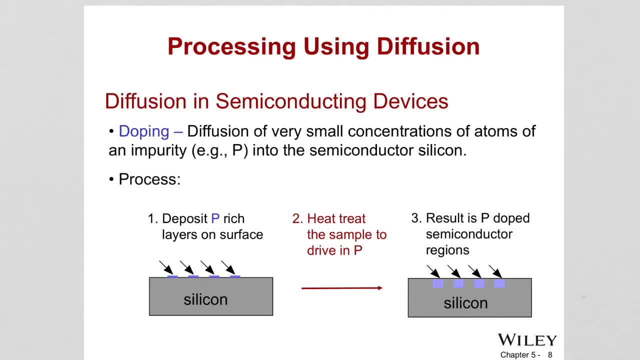 And in this case phosphorus is diffused into silicon, And this is a process called doping. As you can see, phosphorus rich layers are attached to the surface of a silicon And then we heat treat. Of course, there is always heat involved because it enhances diffusion rate. 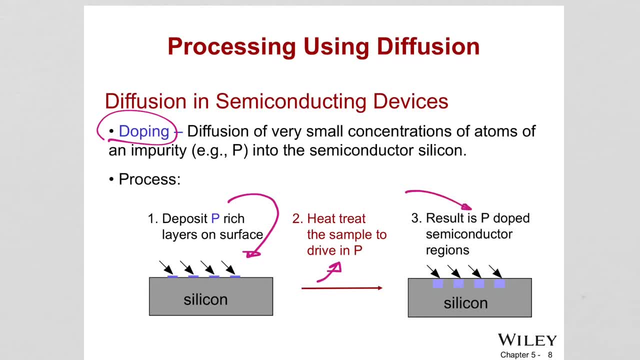 And then, therefore, we are seeing the phosphorus is diffused into the silicon And formed regions, Semiconductor regions, inside the silicon. So this is another technique where the diffusion of atoms are important to understand. What are the parameters that are controlling the diffusion? 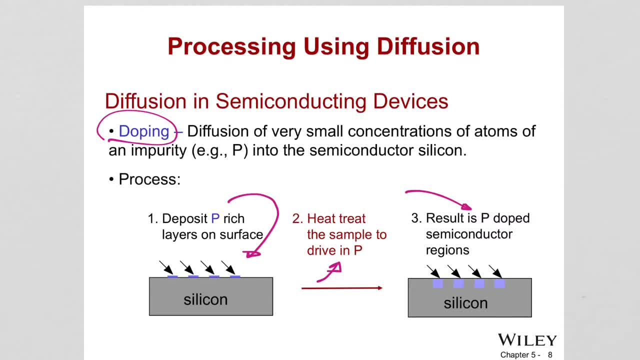 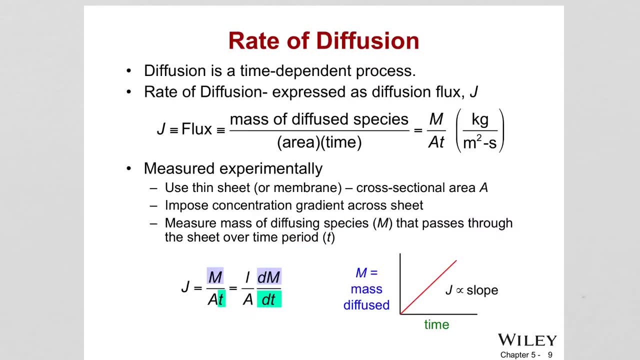 Because these are important to understand when we are actually doing the processing of these materials. Okay, so diffusion is a time dependent process. Of course it will take time for atoms to diffuse from one place to another. Right, And as a function of time, how much they diffused it's gonna change. 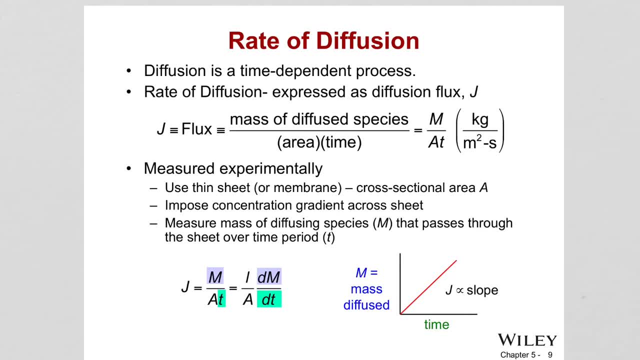 And how do we define the rate of diffusion With a term J We call flux. Okay, So this is in units of mass per area per time. So basically, what is it? Mass of diffused species per area per time. So mass over area time. 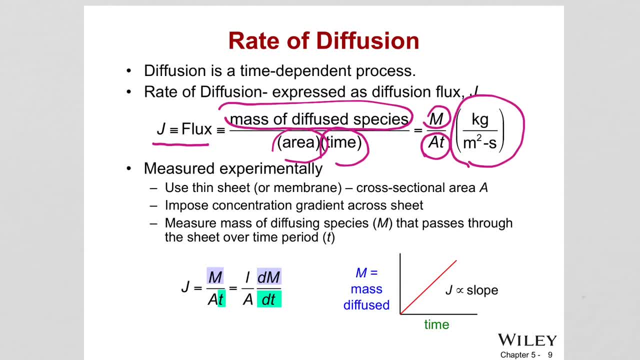 Okay, So this is a very general definition. And how do they measure it? They measure it experimentally. So if you have a thin sheet of material, Let's say like that, And one side you have certain amount of something, It's certain concentration. 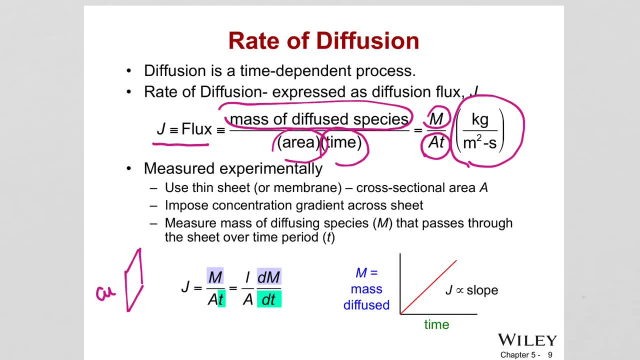 Let's say copper in this side And other side it is zero. Let's say the concentration, So the copper will diffuse through it, Right. And so they measure it as a function of time, How much copper diffused, And the slope of course. 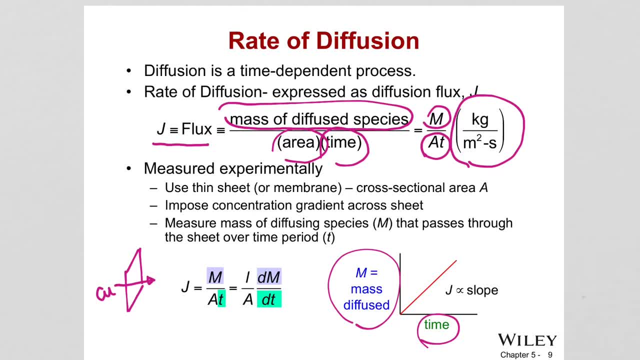 Is gonna give you the flux with the area in formation. This is a fixed area, Right Cross sectional area. Don't worry about this equation here. Okay, So basically, this is a general definition of the rate of diffusion. Basically, It is defined by flux. 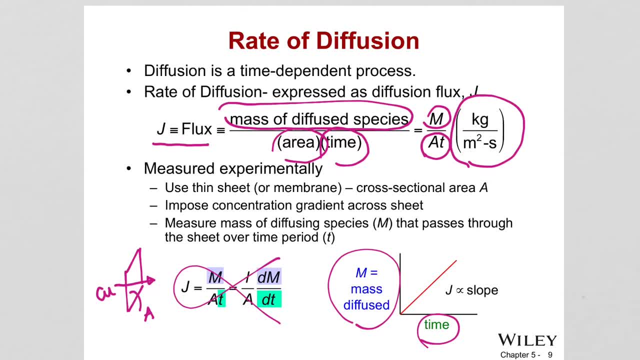 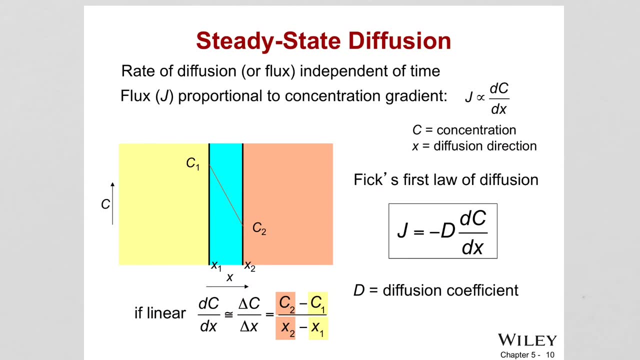 Which is the mass of diffused species per area per time. And how do they measure this? They measure it experimentally To figure out the rate of diffusion. So there are two types, Okay: Steady state diffusion And non-steady state diffusion. 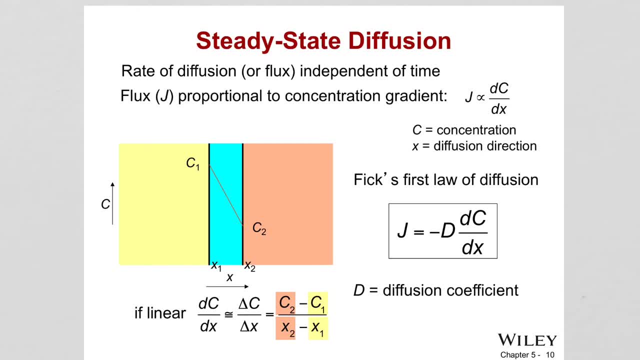 Steady state diffusion is explained by Fick's first law And we gonna see. the non-steady state is for Fick's second law And in steady state diffusion, Rate of diffusion or flux Independent of time, And it is independent of time. 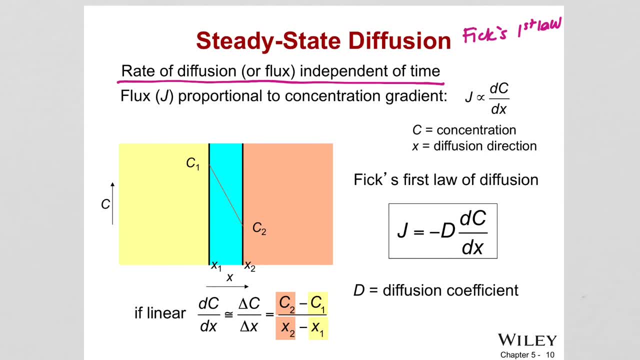 And the concentration gradient Across the material is the same throughout. Okay, So the relationship. it was found How the flux is actually proportional to the concentration gradient. Okay So concentration gradient means How the concentration of diffusing species changes along the thickness. 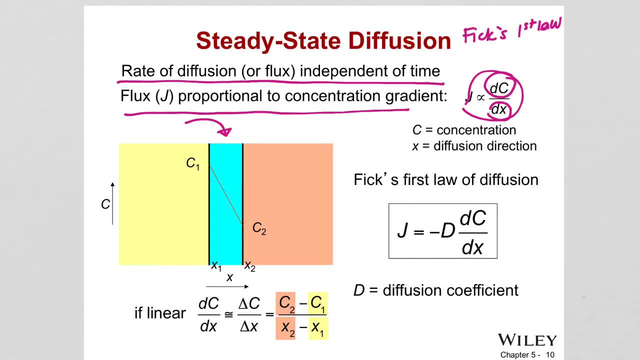 And if you take a look at that, The blue is your material. Let's say At the position, changing from the thickness is changing from a position of X1 to X2. And the distance is the difference you can say is X, And one side of that material we could have a concentration of diffusing species, C1. 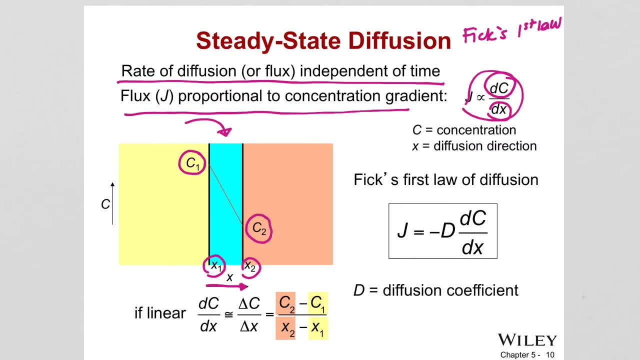 On the other side, it is C2. So C2 is lower than C1. Therefore, From higher concentration to lower concentration, The species will diffuse. And this is showing you, from C1 to C2.. There is a constant. There is a constant concentration gradient. 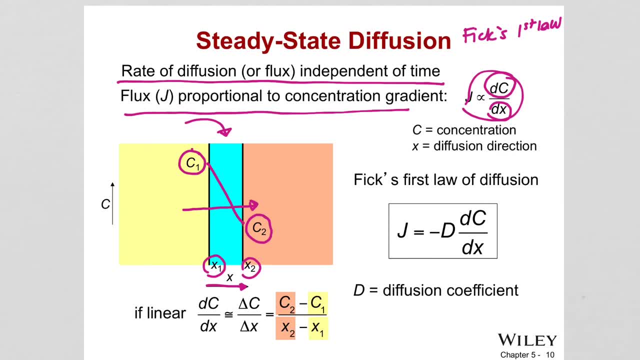 So, Therefore, The expression for the flux, when it is fixed first flow, Is given to us through that equation, Which is: the flux is equal to minus D And times the concentration gradient. And this relationship, This proportionality constant, is actually between the flux. 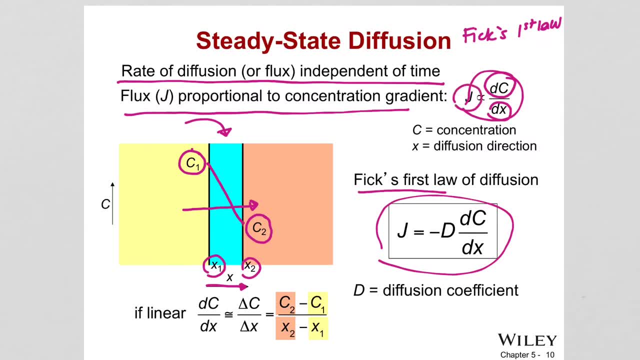 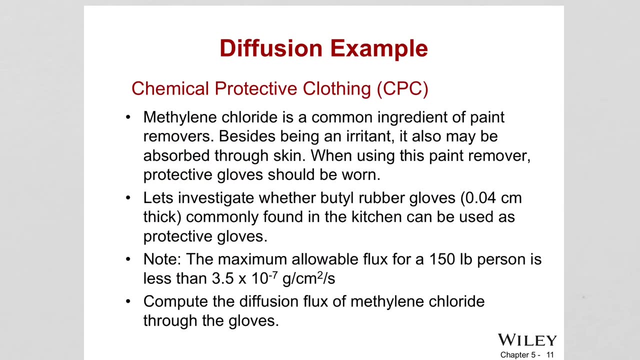 And the concentration gradient is given to us with diffusion coefficient, The expression And the friction is given to us with D. So Depending on that, We can. So let's see this example. We have a metallic chloride Is a common ingredient of paint removers. 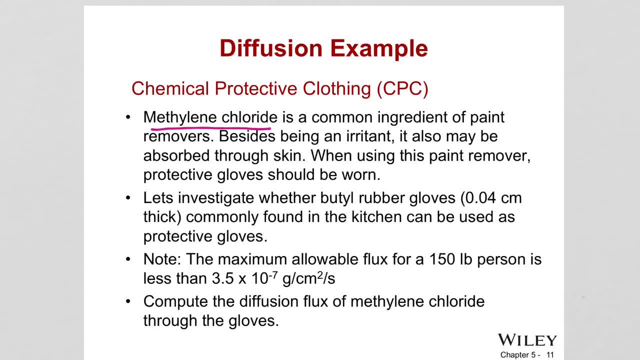 Besides being an irritant, it also may be absorbed through the skin. When using this paint remover, protective gloves should be worn. Let's investigate whether rubber gloves commonly found in kitchen can be used. So the maximum allowable flux for 150 pound person is less than this. Okay, so the flux is. 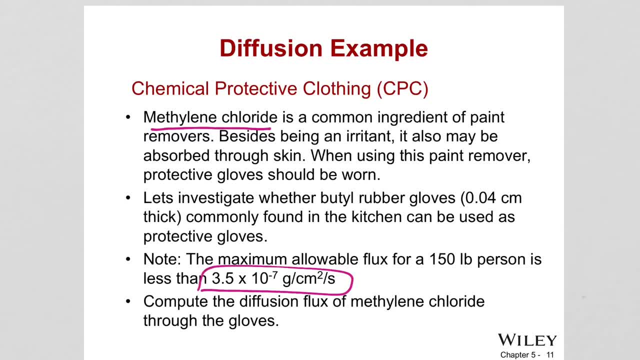 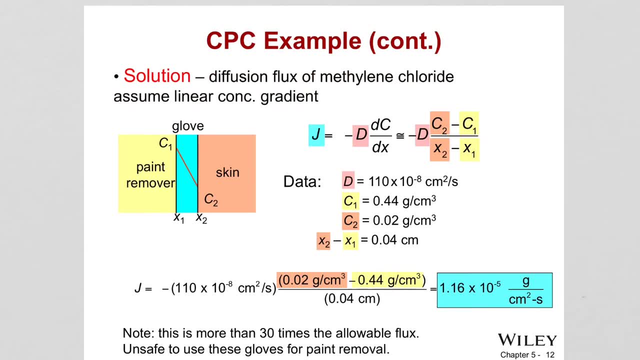 given to us Compute the diffusion flux of metal and chloride through the gloves. Okay, let's compute it. Okay, so the idea here is we have a paint remover which we don't want it to diffuse through the skin. The skin is on the other side. 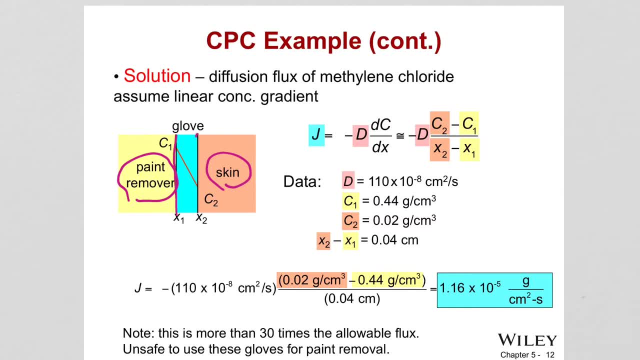 and in the protection we put gloves right. So we need to look at the diffusion flux, or diffusion rate of this paint remover through the gloves into the skin. if this is possible. Okay, because there is an allowable limit. and let's see what is the flux. Of course, certain. 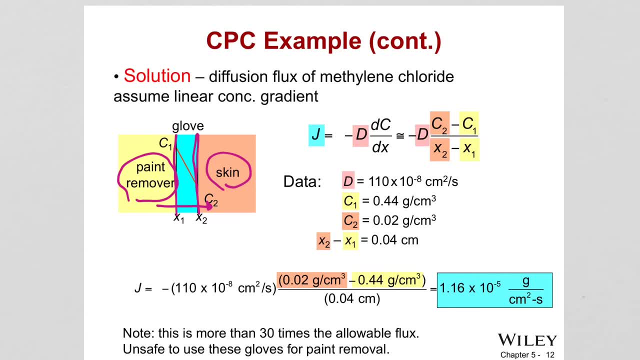 information has to be given to you, right? So by fixed first blow, the flux is minus d times the concentration gradient. Here the minus sign represents diffusion occurs down a concentration gradient, So that negative sign is only for a direction. Okay, since this is c2 minus c1 and we are saying: 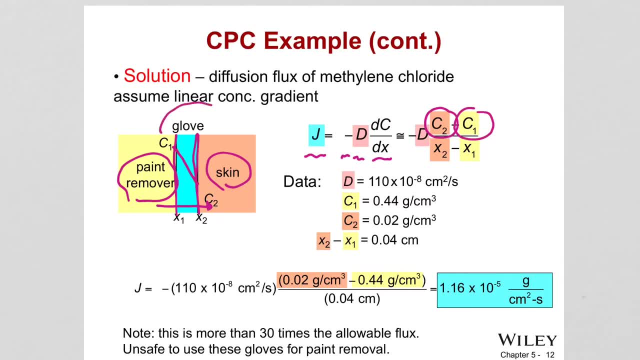 the diffusion is happening from higher concentration, From a higher concentration to lower concentration. that's why there is minus, There is a. the minus is always just an indication of the direction of the diffusion. Okay, so certain things has to be given to us, such as the diffusion coefficient. 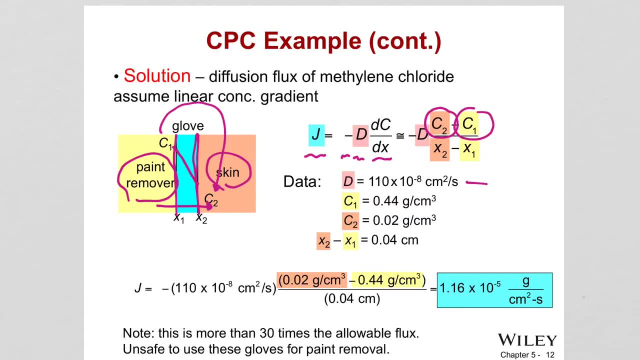 in the units of area per second and concentration difference c1 and c2 of the paint remover on both sides. and what is the? what is the thickness of the glove? this was given to us right, so all we have to do is just plug it in in the equation. basically, we know the diffusion. 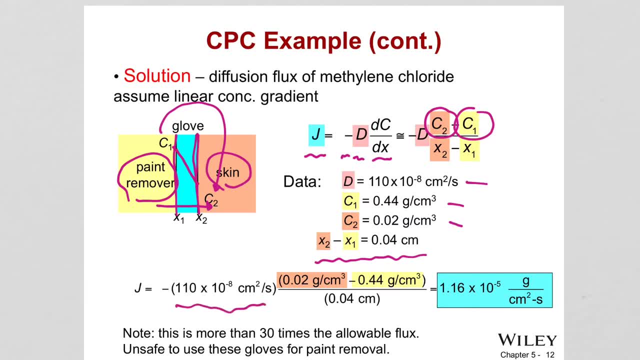 coefficient. we know the concentrations across the glove and then the thickness. look at the units. there are centimeter, good. and then, and when we do that calculation, basically we found this is the flux mass flowing per area per time. okay, so if you look at allowable flux, though, it was right there. 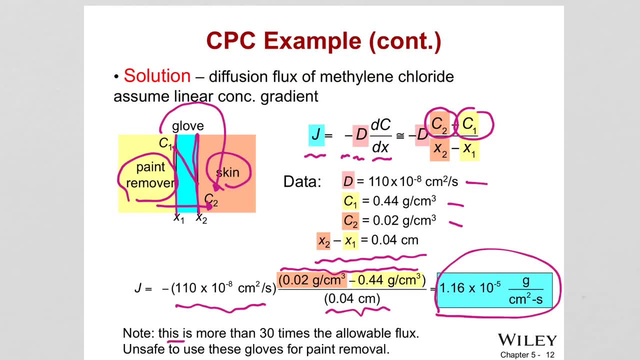 and if we compare it, this is more than 30 times of the allowable flux. so it is not good, right? so this is unsafe to use these gloves for paint removal, so we need to look at other alternatives which will not allow the diffusion of this chemical to our skin. basically, 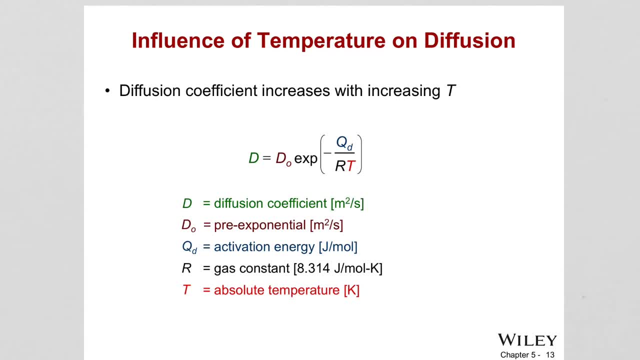 so we have learned: the diffusion coefficient d is in the flux equation right, the rate of diffusion a. But the diffusion coefficient is actually changes with temperature, So it has a temperature dependency And as the temperature increases diffusion coefficient increases. So there has to be a relationship between the diffusion coefficient and the temperature. 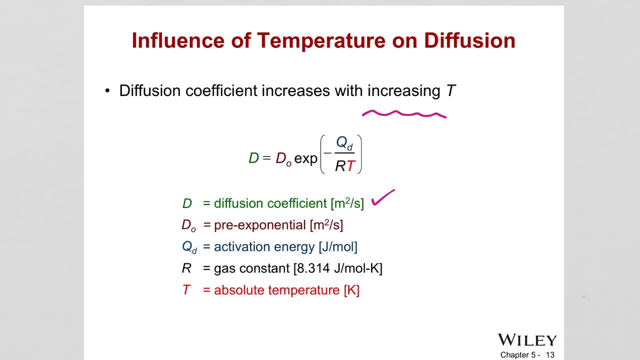 So therefore, through probability calculations etc. there are equations that was found which defines the diffusion coefficient and its dependency to temperature, And that equation is given to us by this equation given here. OK, so the diffusion coefficient is equal to some constant d naught and an exponential term here. 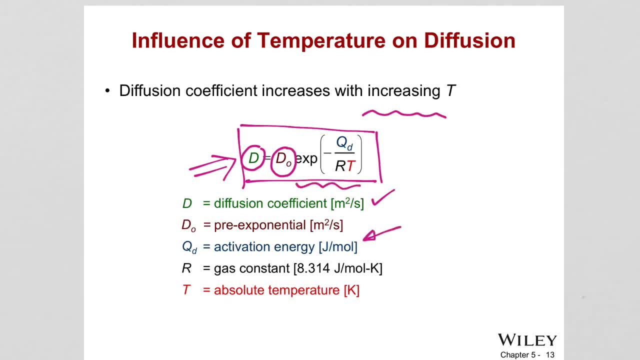 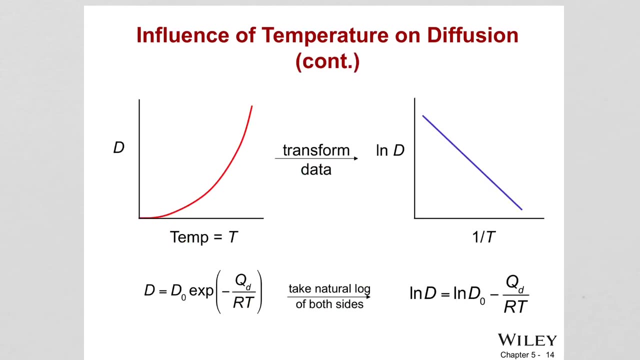 Q is the activation energy for diffusion, And of course there is gas constant R, and the temperature is has to be in kelvins. OK, don't forget that. So if we want to plot that equation, of course d, how it changes with temperature, 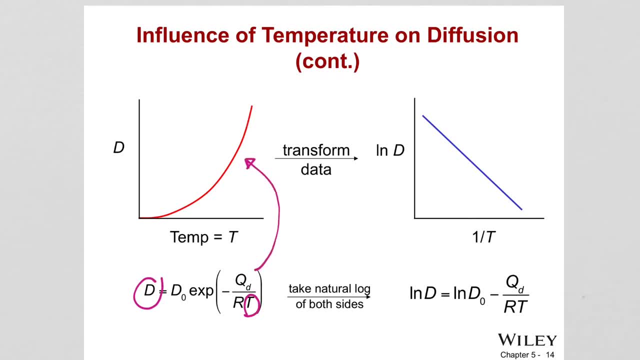 this is the function. This equation is basically plotted in here And we can see how it changes. Of course, it's another linear change If you look at the d and t, But if we transform the data- meaning taking lower rhythms- 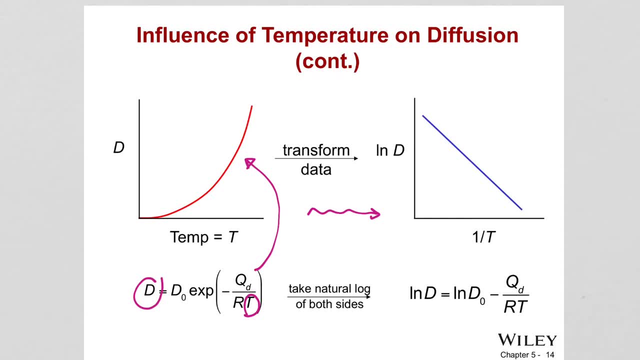 and this will take the exponential term outside of the exponential term. right, This one And, and try it, If we write that equation here, So take the logarithm ln nature, logarithm ln in both of both sides of this equation, Right. 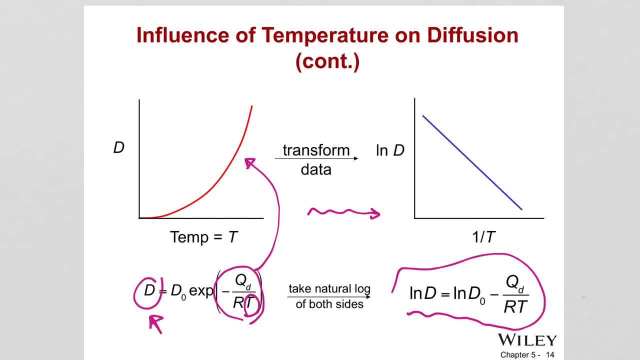 You guys need to understand how to do that Right. This is going to be: and d is equal to ln, d naught minus Of course this exponential term is going to get out Right. It's going to be the activation energy over RT. 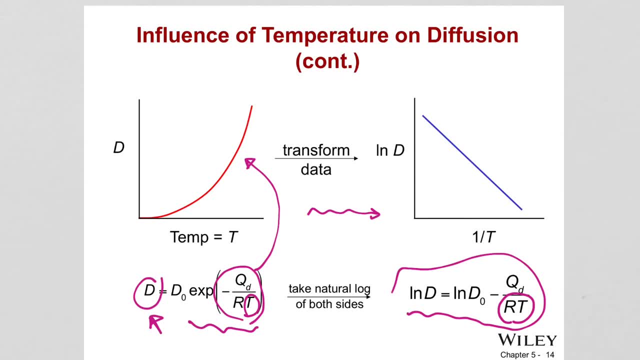 So this is a line equation, Actually, with a negative slope. If you plot ln d, this is y Right Y axis, And if this is your one over, t is here your x. The slope is going to give us activation energy. 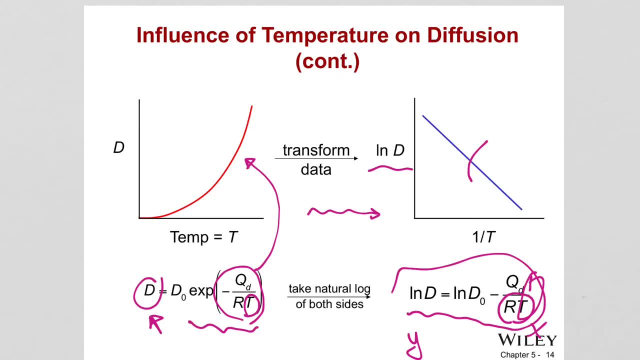 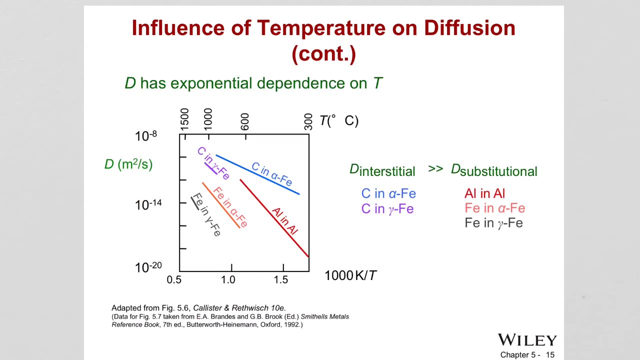 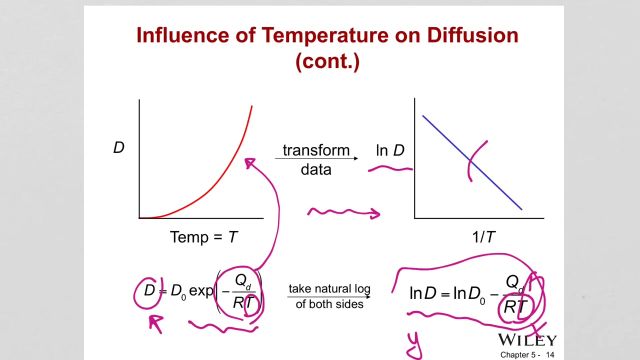 Information Okay, But it is easier in the problems to sometimes work with with the logarithmic form of this equation. Let's see So Okay. So this equation tells us actually with increasing temperature, the diffusion coefficient d is also increasing. 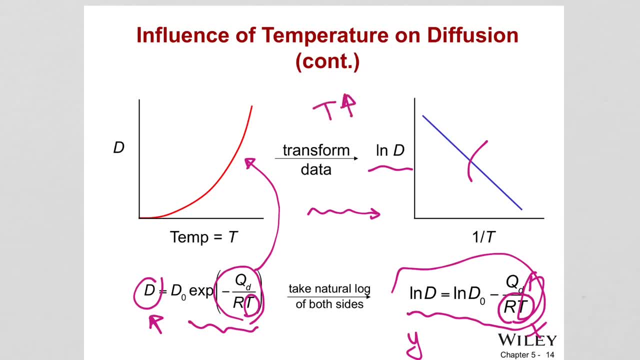 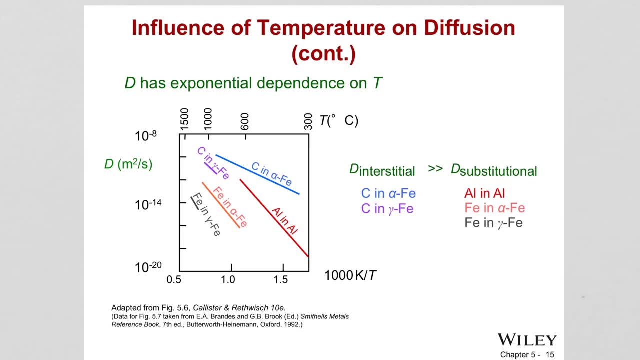 Okay, If we plot this relation between d and temperature, Of course the temperature here This is one over 1000 Kelvin over temperature Here. Basically it is done. It is So. they multiply one over t with 10 to the power of three, because they wanted to write integer numbers here on the axis. 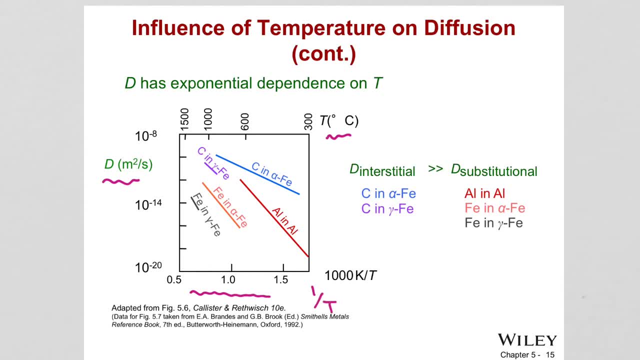 Okay, So normally this is what was one over t, basically times 1000.. Okay, So this way you can write integer numbers For different temperatures, Right, And the temperatures are also shown in the above axis here. Okay, So, as you see, when I move towards this direction, the temperature is actually decreasing. 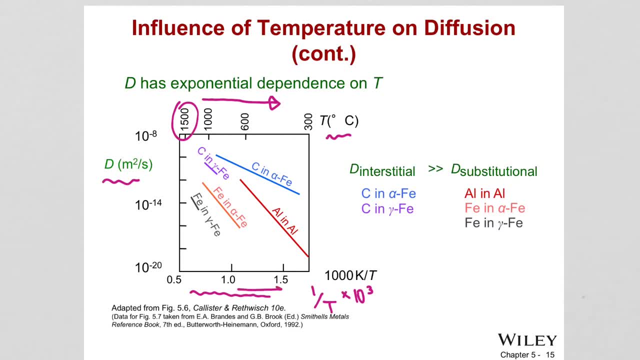 Of course one over t is increasing because it's the reciprocal of temperature. So if the plot The information of diffusion coefficient, there is a diffusion coefficient equation for different systems like the copper, diffusion in iron, aluminum, diffusion in aluminum, that's self diffusion. 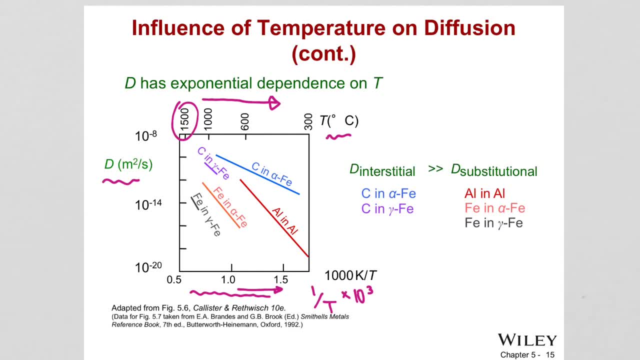 Right, And iron diffusion in different types of iron. So if you experimentally collected data and plotted d versus temperature, what we are seeing here is the thing that I told you guys. So as we decrease the temperature, Okay, The diffusion coefficient decreases. 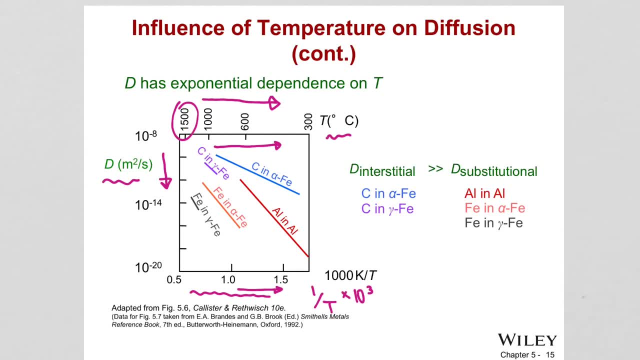 For all types of systems. So, or in other words, as you increase the temperature diffusion coefficient, increases for material systems. Okay, Which is expected, Right? So heat, giving energy to atoms to move around, So which is expected. There is also another information we see. 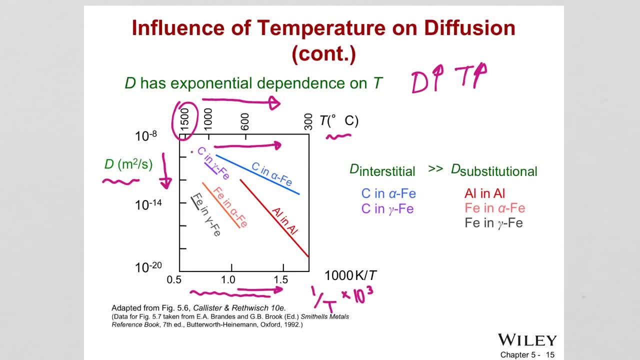 Because if you look at, this is the purple, is carbon in iron. carbon in iron, different forms of iron, Right, Because we learned polymorphism and iron can be BCC and FCC. So carbon diffusion in alpha iron, Alpha iron and gamma iron. 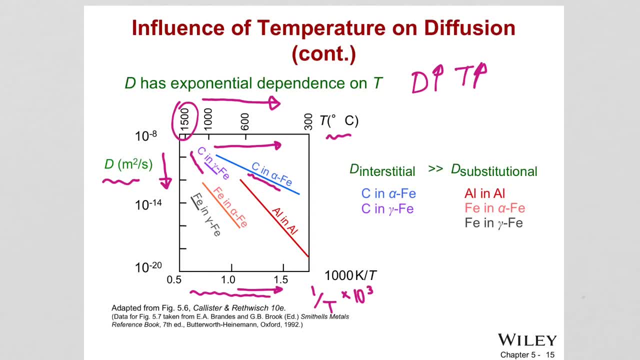 The alpha iron is BCC, gamma iron is FCC. So the diffusion is interstitial diffusion because the carbon goes into the interstitial sites in iron. So when we are talking about self diffusion or substitution, aluminum goes into aluminum spots Right. So iron goes into iron. 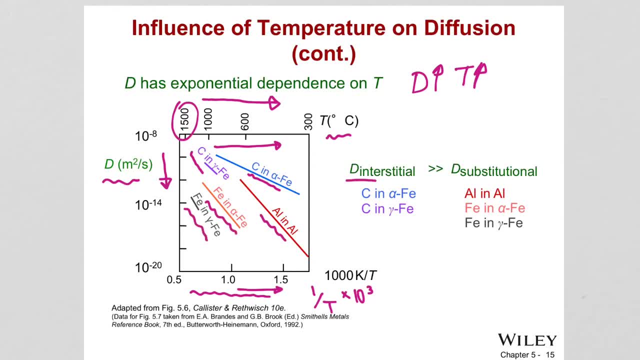 So we can compare the interstitial diffusion coefficients with substitutional ones And we say that the interstitial diffusion coefficient is much higher. Atoms move faster. Right, Because we understand that, because carbon atoms are small in an iron system And we expect the diffusion coefficients to be higher compared to substitutional diffusions. 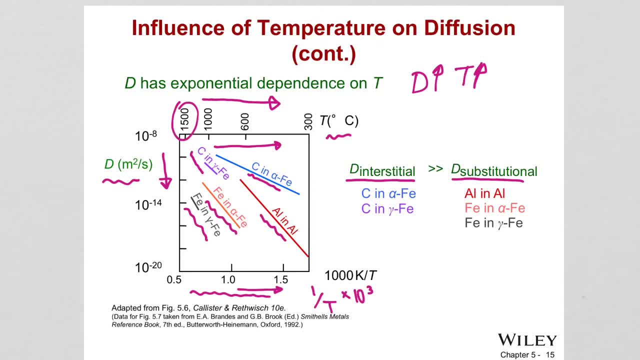 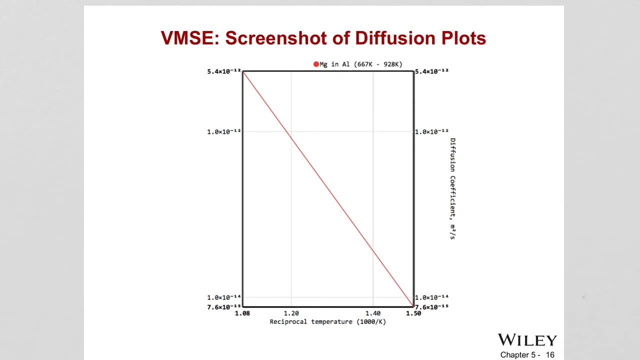 Okay, So this is another information we get. So this is the screenshots of virtual material science and engineering database, And I told you, I gave you the link for this in the pages that I shared with you in Canvas. Okay, So we are given a screenshot of diffusion plots. magnesium in aluminum. 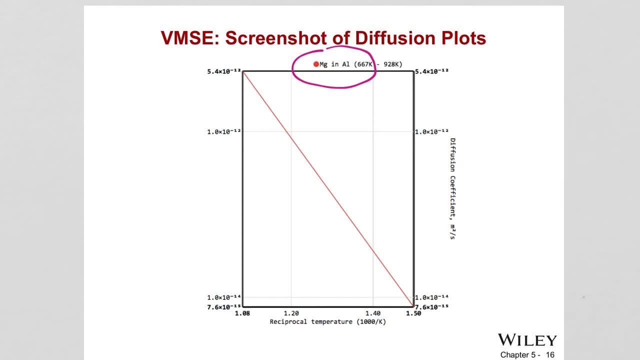 In that software, in that database, if you enter diffusion species and host atoms, some information about diffusion coefficients and activation energies, which we're going to see in the tables next, Okay, And it generates you this plot: basically, D versus 1 over T. 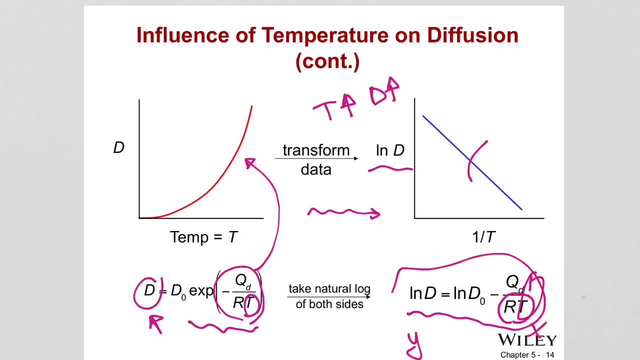 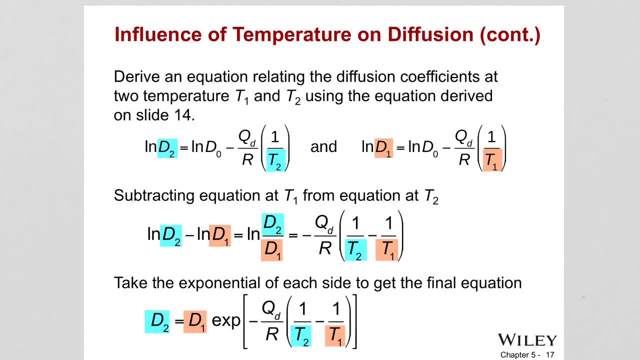 That's it. So this is similar to what we learned here, Right This one. So here we are, asked to derive an equation that relates the diffusion coefficients Of the same system but at different temperatures. So we know that with temperature, diffusion coefficient change. 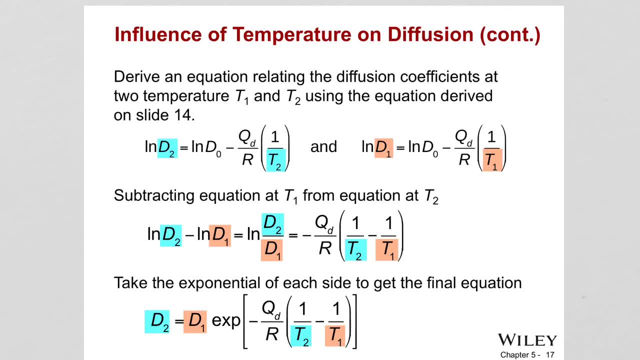 But it goes from, let's say, D1 to D2.. Right, With different temperature, but for the same system. And we are asked: what is the relationship between D1 and D2, basically- And this relationship is going to be important when you are solving equations- 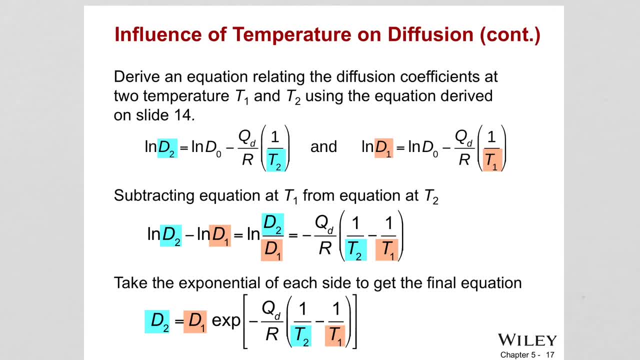 Problems about diffusion. Okay, So let's see how we can derive it. One thing I would like to mention here is that diffusion coefficient depends on the temperature. Okay, And we know that, So, but the D naught. the constant depends only on the system. 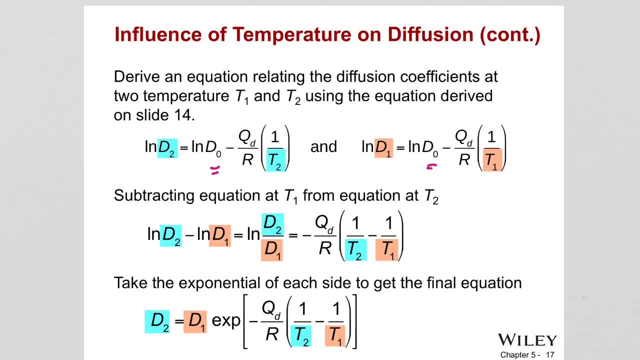 So if your system is the same, D naught constant is not going to change. Okay, So for the same system, If we want to write the basic diffusion coefficient equation, Logarithmic form of that, For the same system but different temperatures. 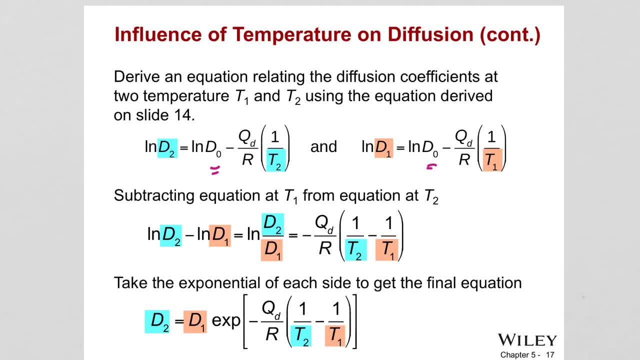 Which are giving us different diffusion coefficients. Of course, we can write this one Right: ln D2 is equal to ln D naught minus Q. So what we are going to do is we are going to write this equation. equation over R. 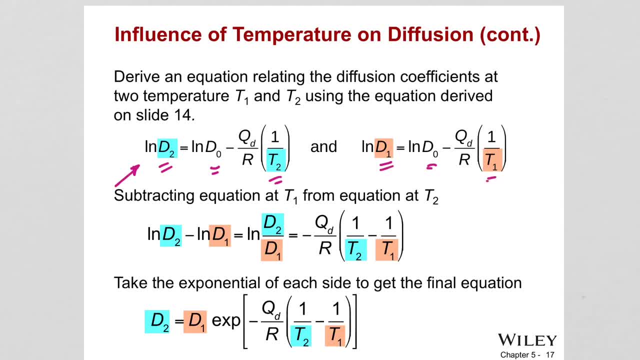 What changes is 1 over T2.. Okay, The same thing. you write it for the another diffusion coefficient of the same system. So if you look at both of these equations and actually Sold it for ln, D naught because that's the same in both equations and has to be equal. 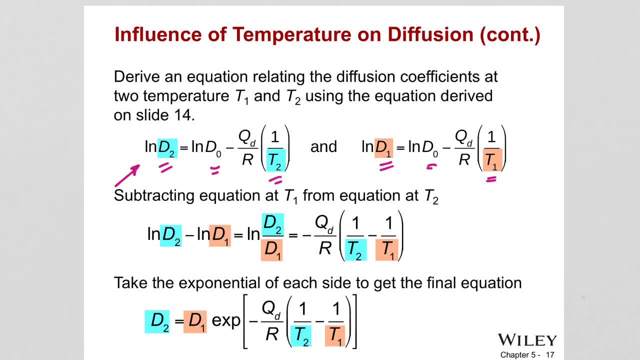 To each other, Right? So let me try to do it here. And of course, activation energies are the same. okay for one atom to move from one place to another place. So I solved both equations, for ln d0 and ln d0 is the same for both equations. 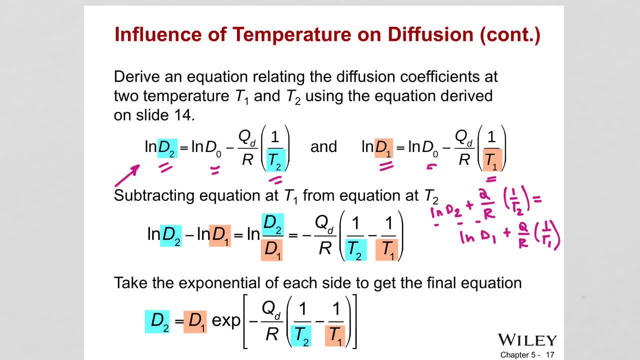 So that means this term here has to be equal to this one, and this cancels out d0, right, We don't need d0 anymore here. So if we again rearrange this, this is how it's going to look like, right? 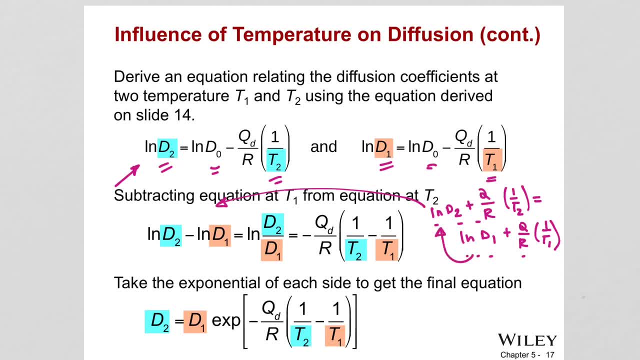 So this comes to that side: ln d2 minus ln d1, which is equal to. also because this is a minus sign and because of the properties of ln, we can- instead of minus we can- write ln d2 over d1.. 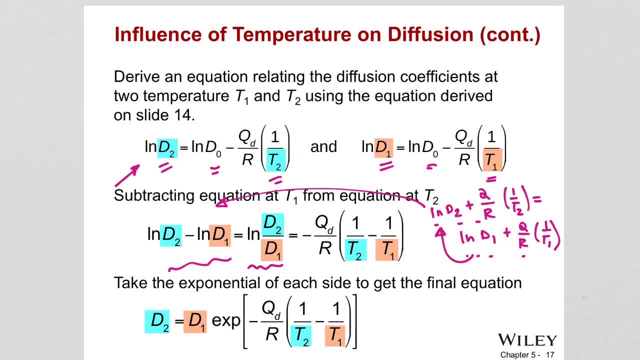 That's fine. And then we have, on the other hand side, the q over r. parenthesis is possible because the q over r is the same. So it's going to be 1 over t2 minus 1 over t1, with the negative sign here. 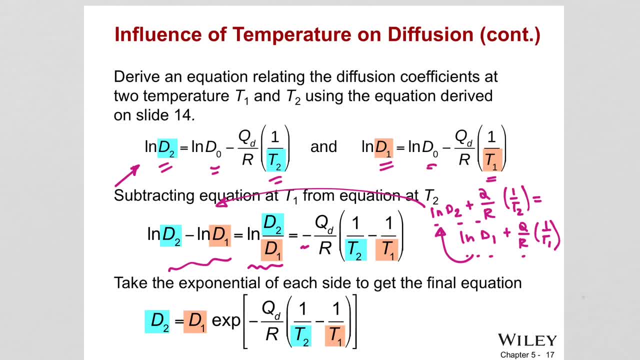 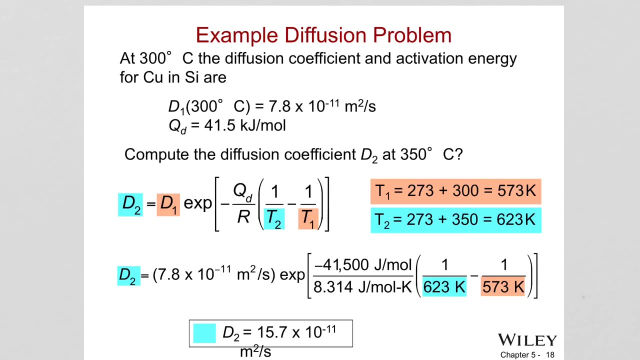 You can also write it. if you want to write it in the exponential form, You can also write it this way. Okay, now let's solve a problem, since we derived the equation which relates the diffusion coefficient of the same system at different temperatures. Okay, so let's solve it. 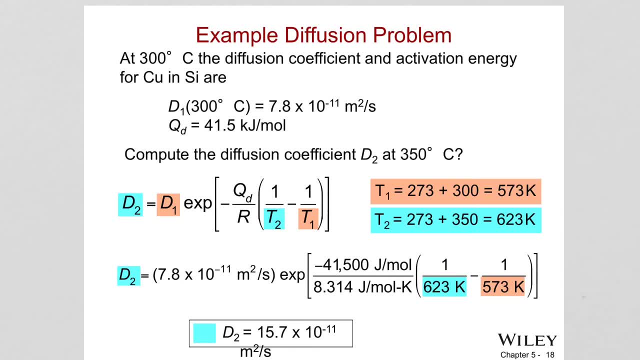 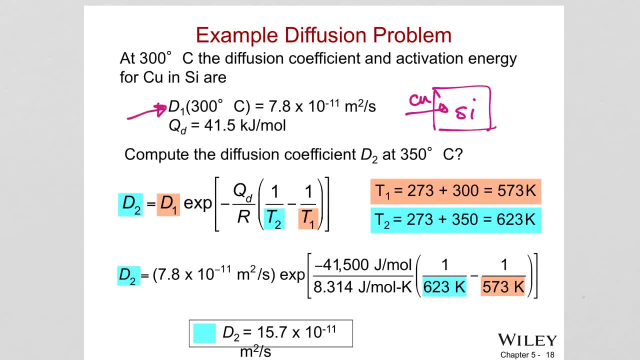 And diffusion coefficient is given. of course it has to come with the temperature, because the diffusion coefficient changes with temperature, right? So at 300 degrees C we are given the diffusion coefficient. is this. So sometimes it might not be given like this, but sometimes you might need to read it from: 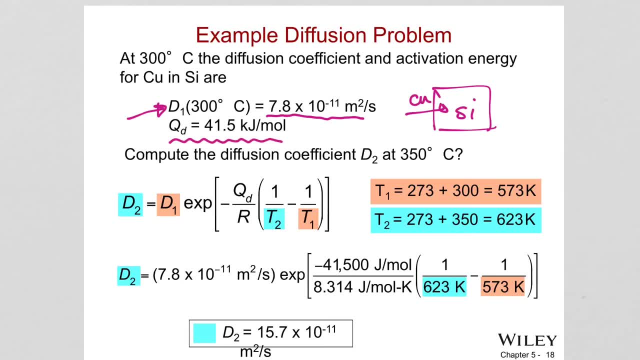 a table And also the activation energy for the copper-silicon system is given, It doesn't depend. It depends on the temperature, It depends on the system. So compute the diffusion coefficient at 350.. So we are given the diffusion coefficient for a system at certain temperature and we 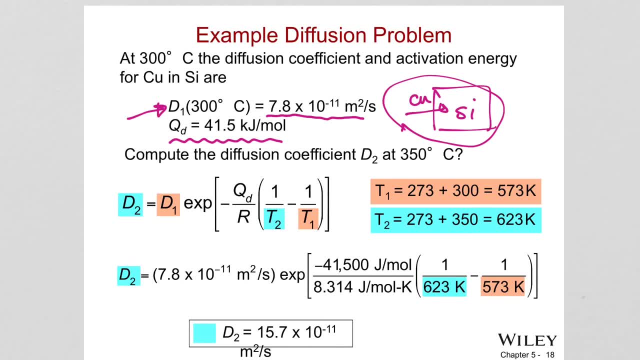 are asked for the same system. what happens if we change the temperature? how the diffusion coefficient changes and we now learn that there's a relationship between D2 and D1, and it is given from this equation. So all we have to do is plug in the information we are given. 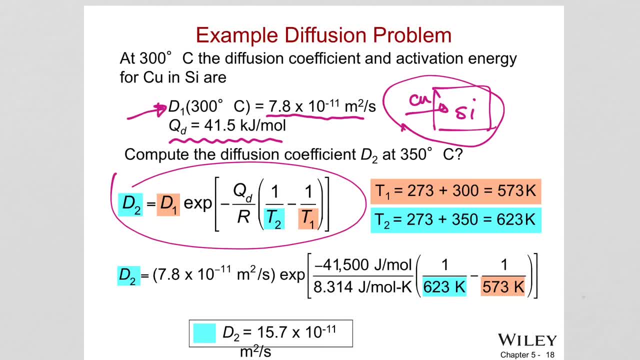 So the temperature has to be Kelvin. So change those to Kelvin and plug it into your equation. R is a constant which is given, And Q is given. You need to be careful with what is the unit of R. Since the unit of R is joules, it includes: 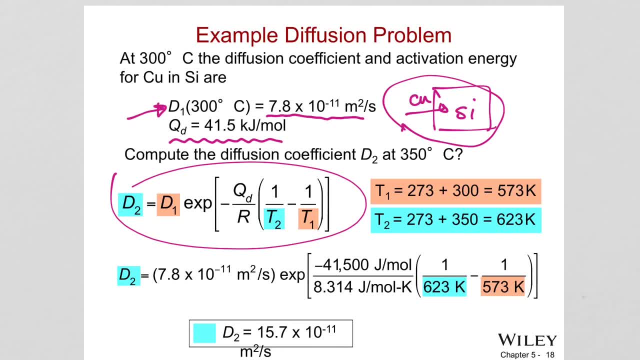 joules. So unit of the activation energy should be converted from kilojoules to joules, So you need to be careful in those units. And then diffusion coefficient at D1: for D1 is given, Plug it in And basically calculate what to expect in terms of the diffusion coefficient at a higher. 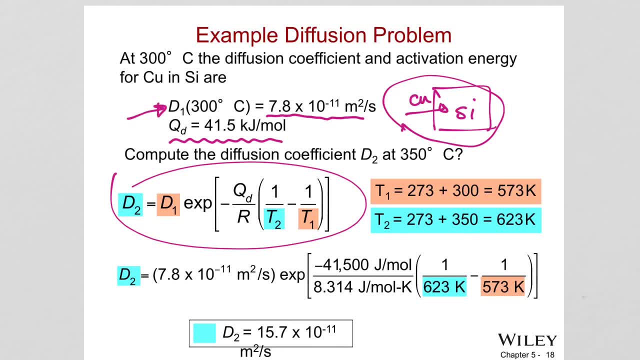 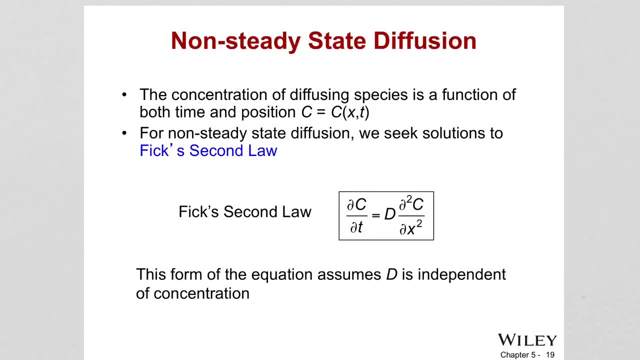 temperature, which we expected to be higher. So, if you compare D1 and D2, you will see that D2 is higher because it is an increased temperature compared to 300.. Now we are at 350.. Okay so, as I described to you guys, there is steady state and non-steady state. 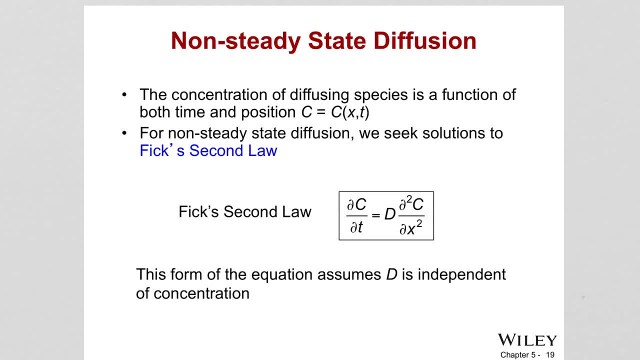 In the steady state, the concentration gradient across the film, across the thickness, was the same. Okay, Okay. So in reality there are situations where that concentration gradient is not going to stay the same because, as the species are diffusing from one point to another, the concentration 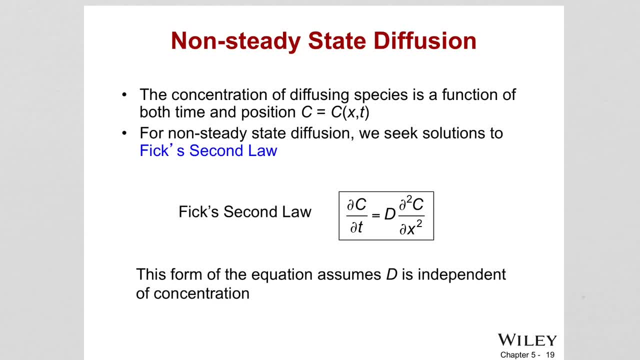 on both sides of a thickness basically, will be changing with time. So therefore non-steady state diffusion is happening if the concentration of diffusing species is a function of both time, Time and position. So C, the concentration of diffusing species, depends on X, the position, and T is the time. 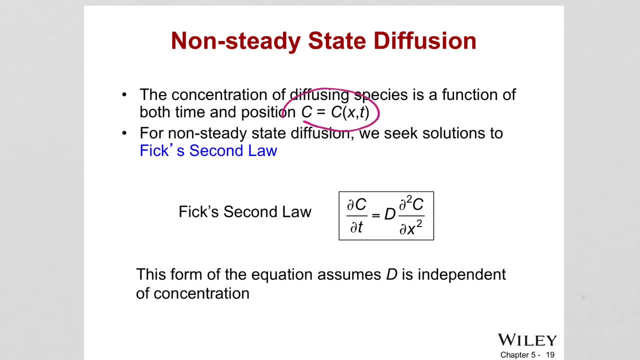 Okay, So we are writing it. C is a function of X and T, So this is defined with fixed second law equation And you can see in the equation The dependence of the concentration to time and the thickness The time is included in that equation. 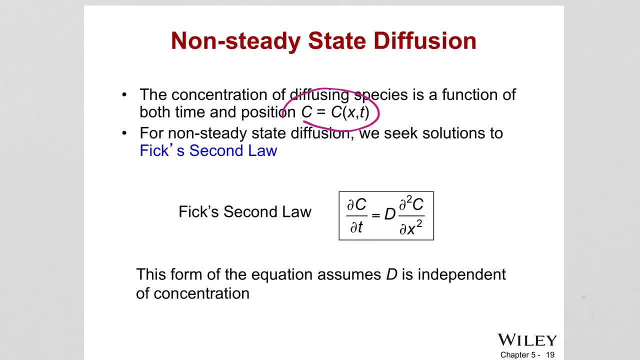 And so in this form of equation, the diffusion coefficient is of course independent of the concentration And it is defined as the same way, right, The D is depending on activation energy. It depends on the type of system, basically over the temperature. 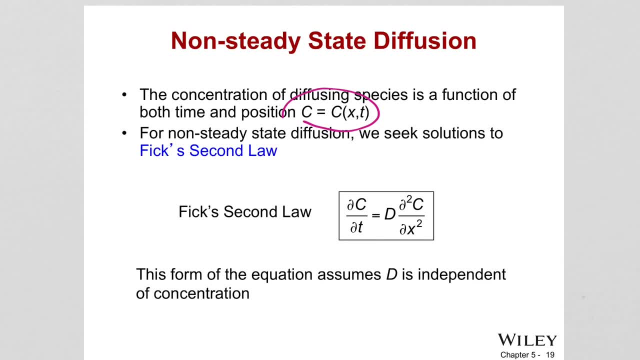 So this is how the fixed second equation is given here. What does it say actually? The rate of compositional change is proportional to the rate of change of the concentration gradient, rather than the concentration gradient itself, Like it was in the fixed first law. okay, 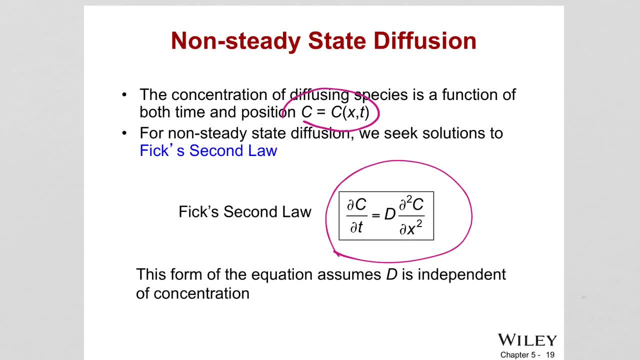 So this is a differential equation and we need to solve it. okay, So how do they solve it? They need to define some boundary conditions to solve this equation And relate the concentration, time, thickness and diffusion coefficient. okay, So, as I said, to solve this equation, basically we need boundary conditions. 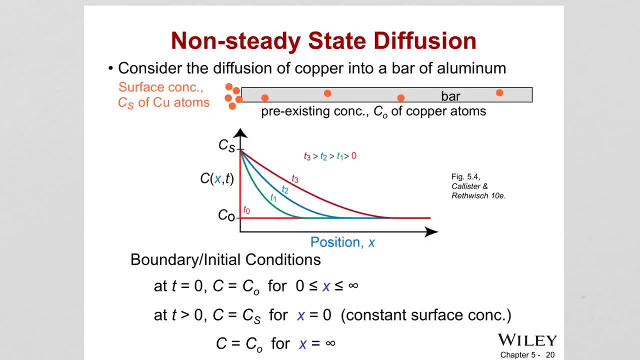 Okay, let's see. So how does these boundary conditions gonna be defined? okay, So we have some definitions here. Let's consider the diffusion of copper, shown with the orange dots here, Uh, into a bar of aluminum. Okay, here is the bar where you are seeing, right there. 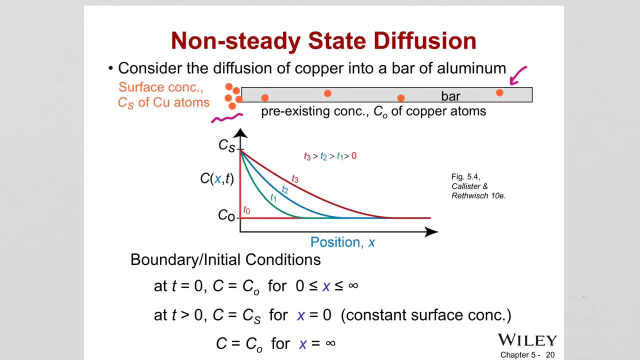 Okay, So first, what is the preexisting concentration of copper atoms in the bar C-NOT? right, C-NOT is gonna be defining, uh, what is the initial concentration of diffusing species, The copper? What is it? 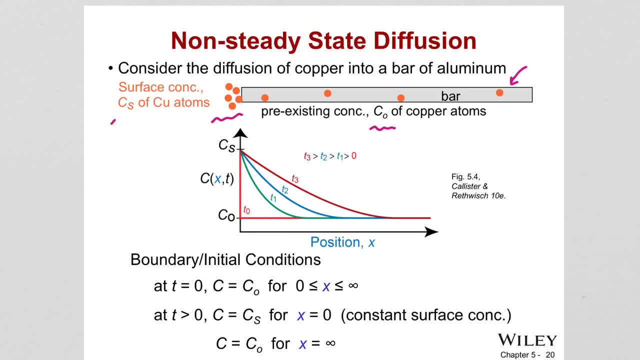 Right, And CS C with a subscript S is the surface concentration of copper at the surface of the aluminum. Okay, so if we look at time 0, the concentration which depends on remember x and time, and the concentration is equal to C0 at time 0.. 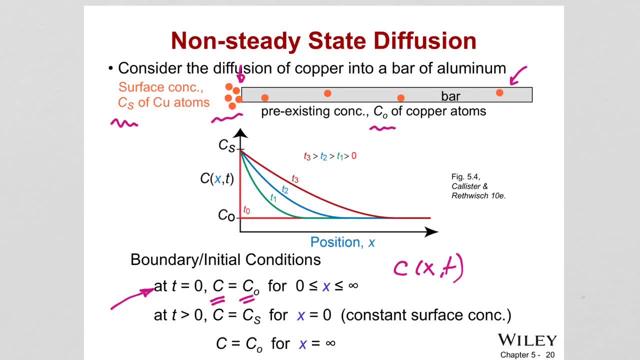 Because at time 0, we know the concentration of diffusing species in the bar is equal. So at a time that is bigger than 0,, when x, when we are at the surface right, when x is 0, the concentration equals to surface concentration. 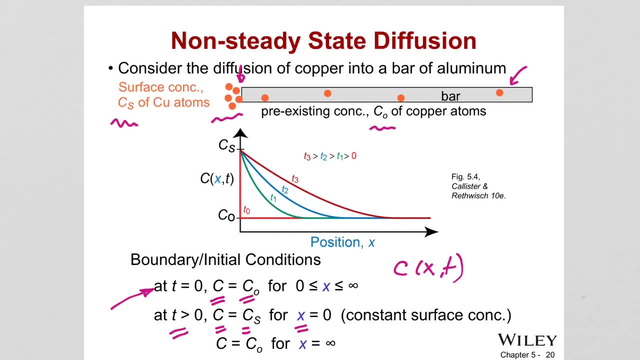 At a time bigger than 0, when we are far away, x is infinity. right Far away from the surface, the concentration is going to be equal to the initial concentration. Far away, right, Far away. Okay, so these are defining boundary conditions to solve that differential equation. 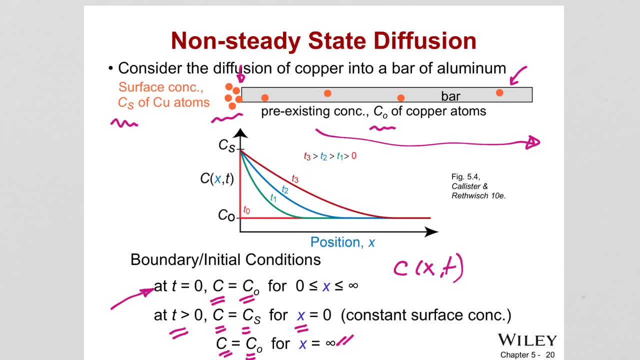 Okay, that's it. Of course, also, if you look at this figure, we are seeing how the time is important In terms of understanding the concentration change with time of the copper diffusing species. So, at a time 0 and x0, when we are here, we are seeing that the concentration is actually C0, right. 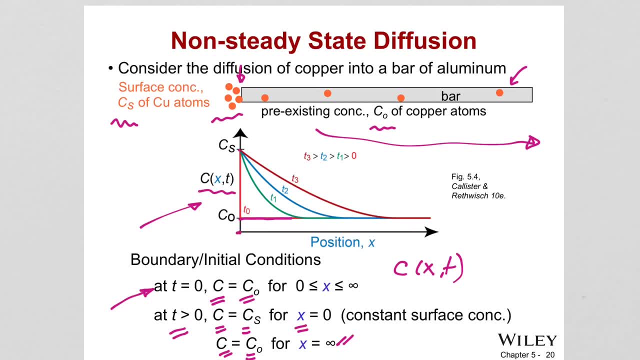 But with time it is starting with Along the position of the aluminum. of course we start from here and move along the bar. okay, So we start. the concentration starts at the surface with Cs and as we move along the bar it is actually increasing. 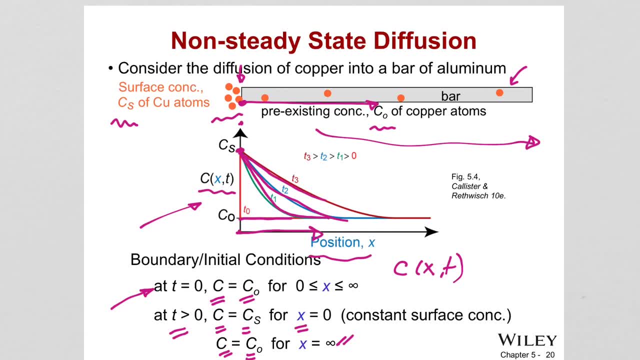 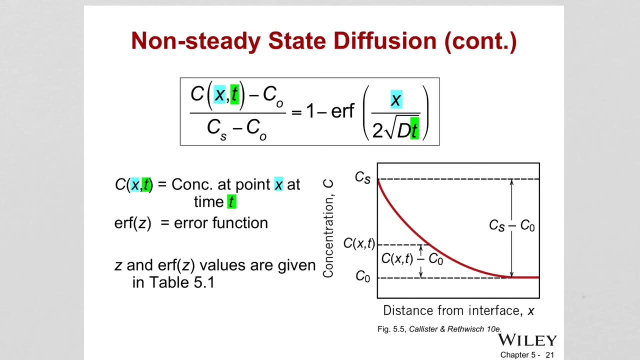 Increasing concentration with increasing time. okay, So at this, At this position, for example, you see that with time, the concentration of copper is increasing. Okay, So we don't have to worry about how this equation was solved, given the boundary conditions, because we are given the solutions of it, okay. 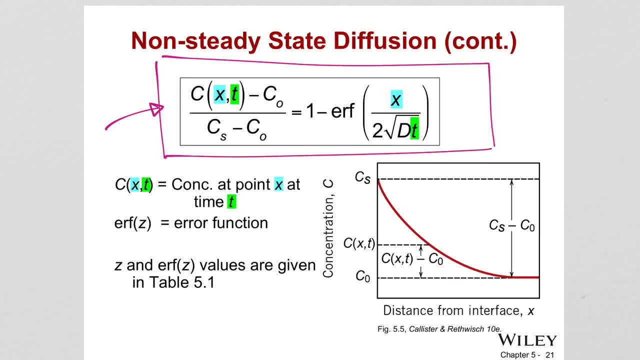 So how this concentration Changes relate to time and thickness, how it depends on it, And that is when we solve that differential equation. this is the solution that we are going to use. So this is the solution of Fick's second law. 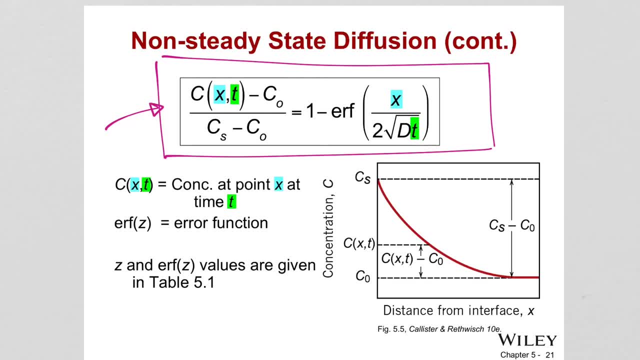 If we look at the terms in the equation, the C has a function of x and t. It is defining us the consumption, So the concentration of the diffusing species at any point. x- at any time, So any point along the bar right. 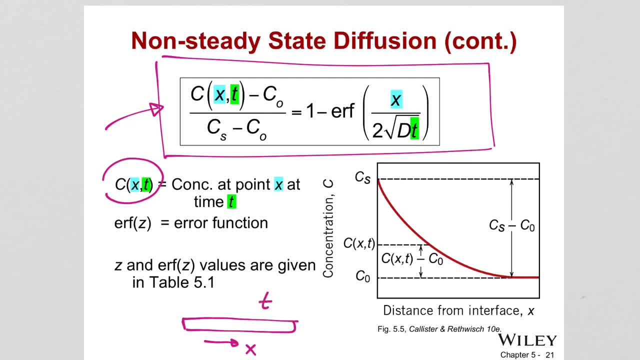 At any time we are. let's say at this point, it's some five seconds later- what is the concentration of copper? let's say, okay, That term is defining. So there is error function. This is general error function. 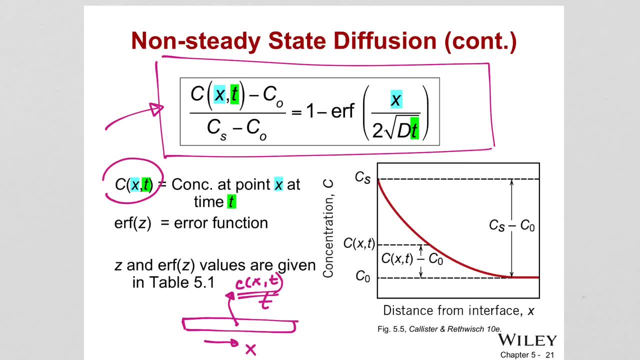 Which the solutions are found in literature. Okay, So this error comes from the way we solve the differential equation. So it is some mathematics, okay. So we don't have to worry. All I need to tell you guys this error function is found from tables, okay. 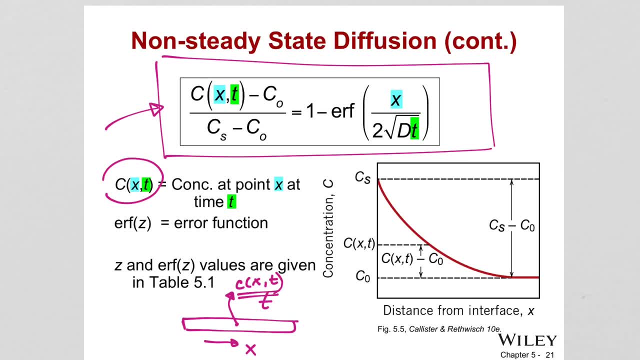 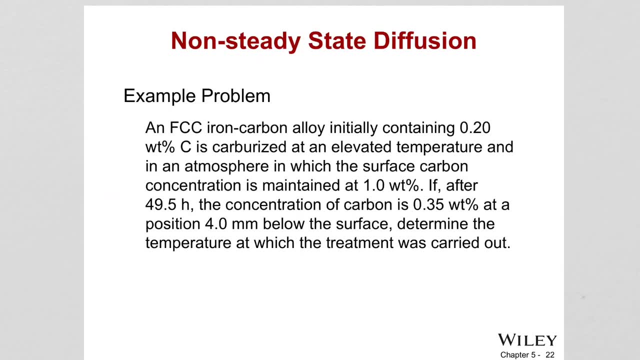 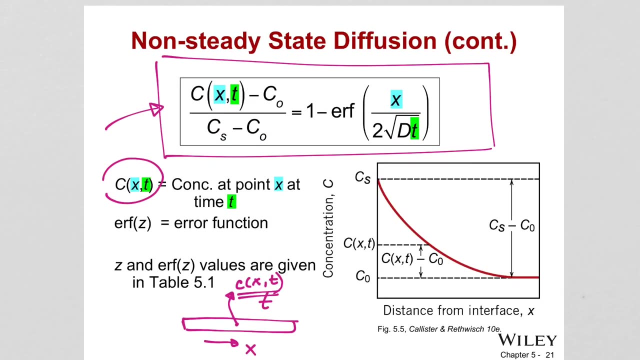 So it is said that z and I mean inside error. So the error function and the error function will be given to us in table 5.1.. Okay, So I guess that table is in our book, But anyhow, we will use it in the problems. 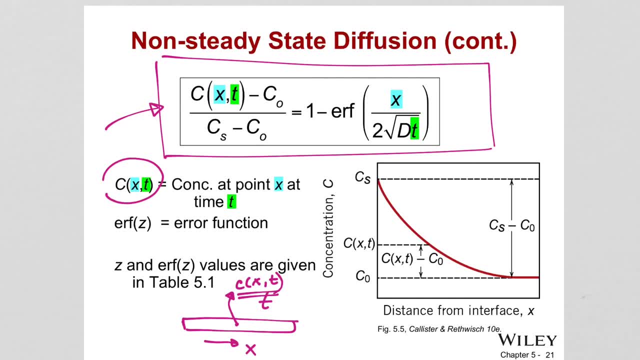 And then I will also. yeah, So I saw that in your book. table 5.1 is giving you error function. And then you don't even need that, You can google. And you, what is the error function? 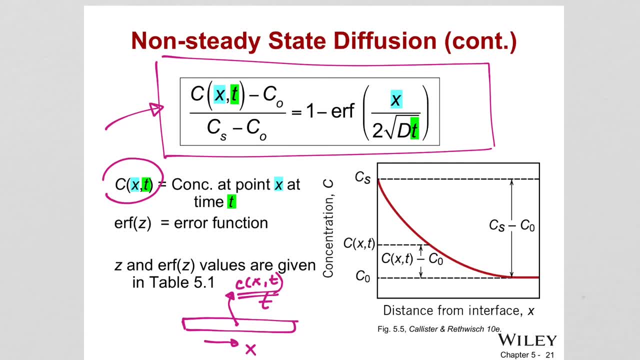 And you can see the images that you can find error function there, And then we're going to do examples to understand that. So if we want to see in a figure how, in a chart, how this equation is plotted actually, 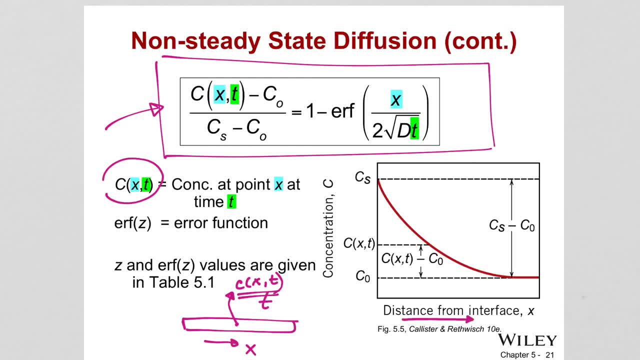 as a function of distance from the interface. Okay, So, starting from here And moving inside the material bar, How the concentration is changing of the diffusing species. It starts at the surface. with the surface concentration As we move inside, it is of course decreasing with distance. 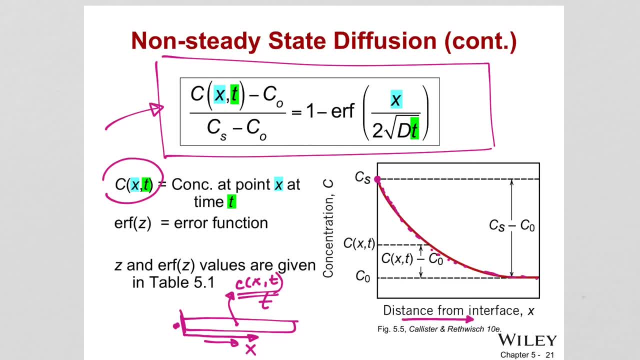 And it also depends on the time, right. So at a certain distance, let's say this point- We will have a concentration. We will have a concentration of those species at a certain point, at a certain time. The initial concentration of these species. within the bar, we achieve it far away, right? 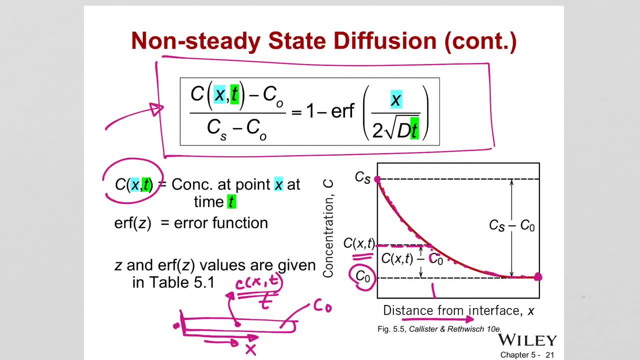 Because the far away we are, so far away from the surface, We are still preserving the amount of initial concentrations inside of that diffusing species inside the material And usually this can be zero right, Because initially there might not be any of those diffusing species. 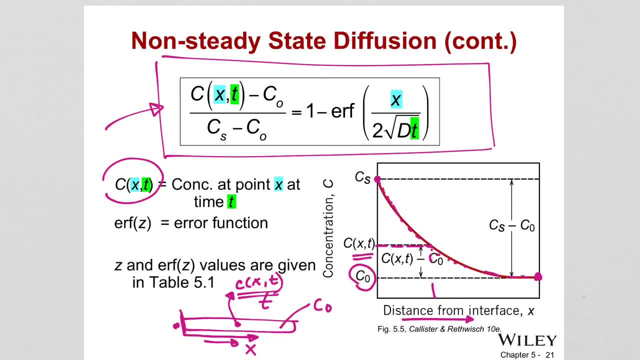 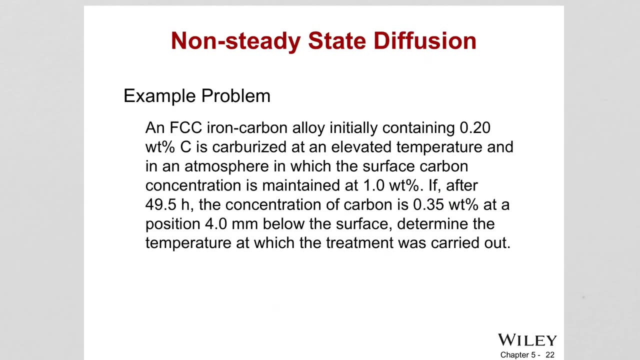 Unless you are diffusing carbon into steel, Because steel already has carbon inside And so you start with some certain C-nut volume. Anyhow, let's see a problem. An FCC iron carbon alloy Initially contain 0.2 weight percent. carbon is carburized at an elevated temperature and in an atmosphere. 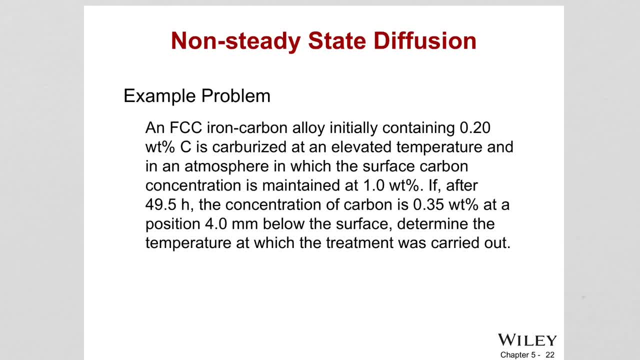 in which the surface carbon concentration is maintained at one weight percent. so we are given, so there is a alloy right and carburized mean, the carbon is introduced, so carbon is diffusing. so of course it has some surface concentration of the carbon and it has some initial concentration. 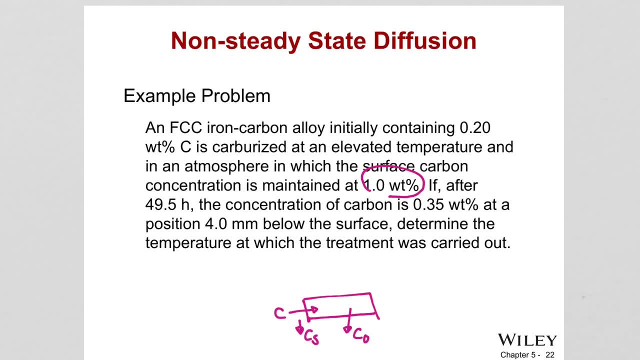 so we are said that initially, of course it has some iron- 0.2, that is given to you, right. and then the surface concentration is maintained in one percent. so after 49.5 hours- so the time is given to us- the concentration of carbon is 0.35 at the position, 4 millimeter below the surface. 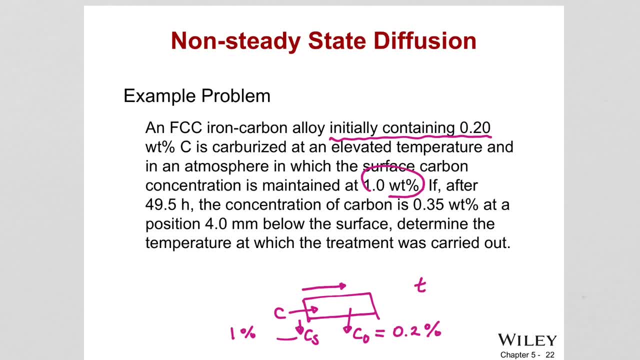 so you move 4 millimeter below the surface, come here and at the time, 49.5 hours, 4 millimeter in depth, we have a concentration of carbon that is 0.35. this is giving us the concentration at a certain distance, at a certain time. 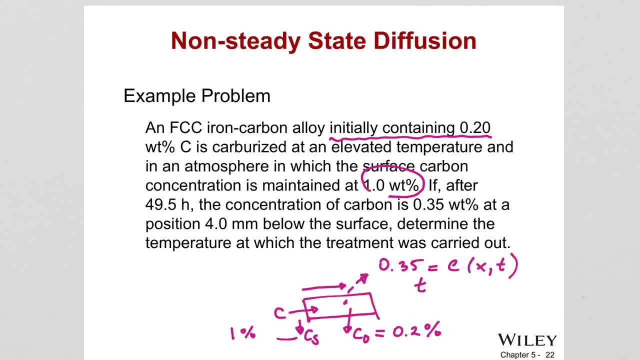 now determine the temperature at which the treatment was carried out. so we are asked: temperature? okay, now let's look at this is first of all you need to understand. this is a fixed second law problem problem. okay, so there is time in it. so when the time is in the problem, that means we are talking about fixed second law. 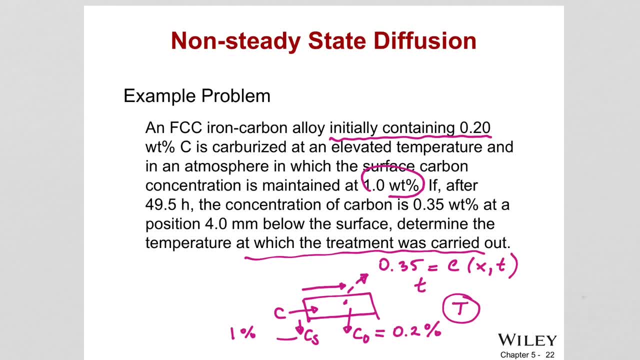 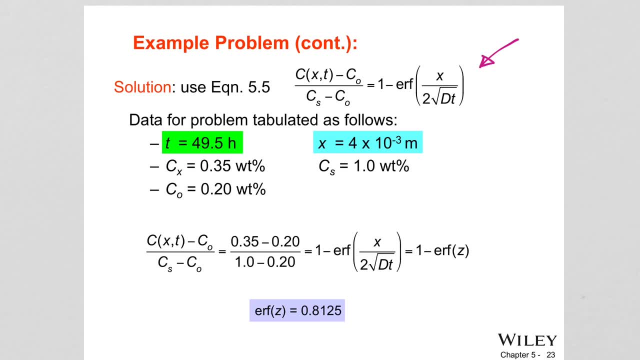 and we are given enough information to plug it in into our fixed second law equation. but wear does this. so we need to solve it with temperature right for temperature. but wear does this. for temperature information coming from, you'll go to remember, diffusion coefficient depends on temperature right. so first we need to solve this to figure out the diffusion. 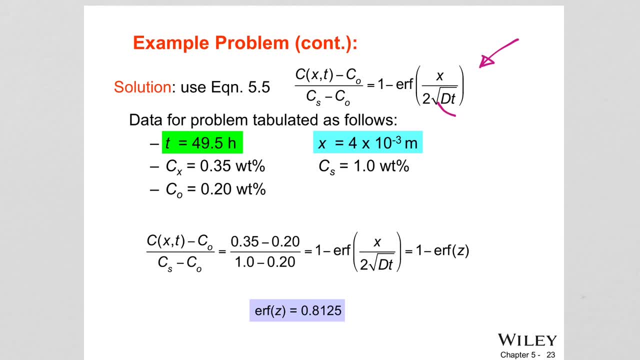 coefficient, and then we remember how many diffusion coefficient is related to temperature, and from that equation I can find the temperature. so our fixed second law equation is given the solution. now all I have to do is plug in the information that we just figured out from the problem. that is given in the 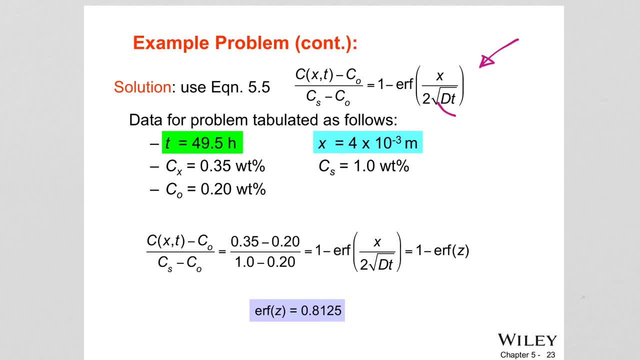 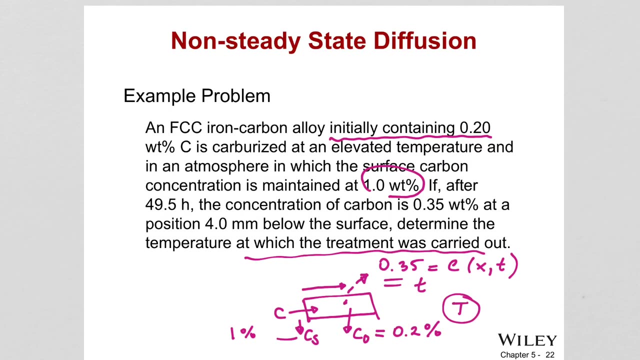 problem and then calculate the equation. basically, let's see what we can we gonna do, okay. so we said concentration at a certain time, certain distance was 0.35, so we put it there and initially the carbon concentration was 0.2. just put 0.2. so all units are the same. you don't have to deal with any. 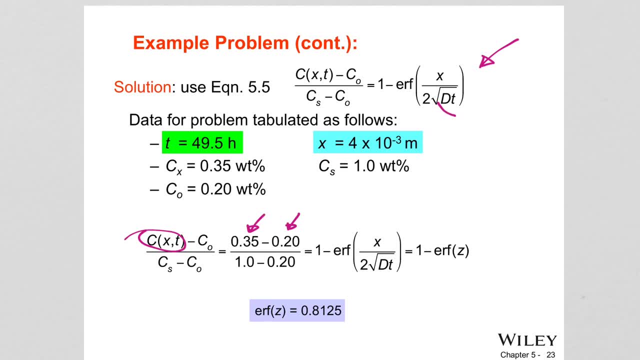 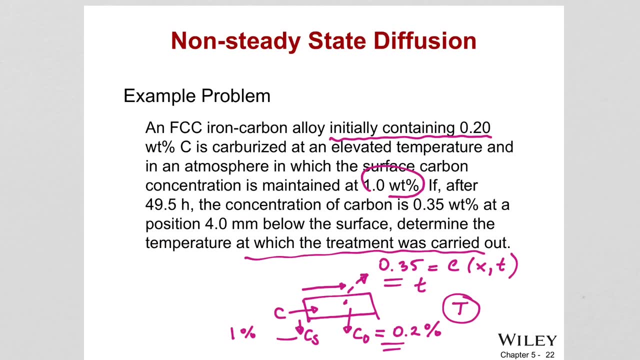 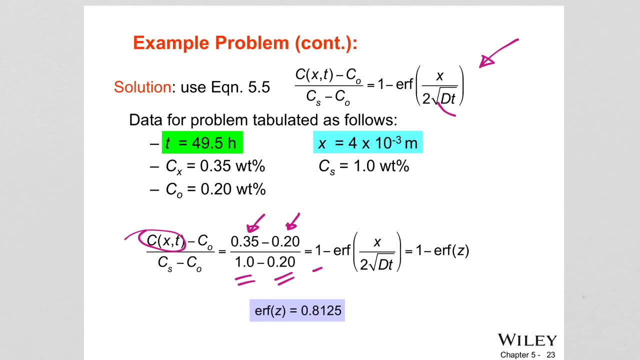 other thing, just put 0.2 right. so all of these are percentages. so as long as the all units are the same, you're fine. so in the surface concentration is 1%, so put 1 and CNOT is again 0.2, which is equal to 1 minus. 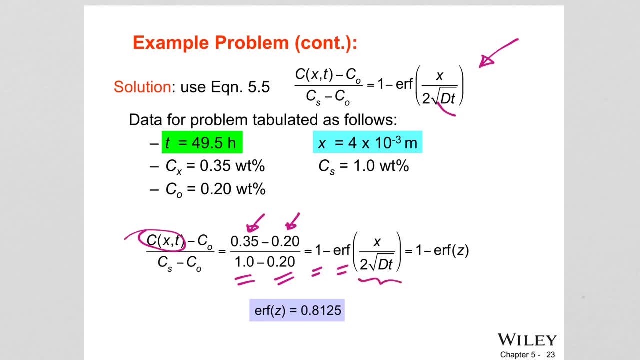 error function and with inside the error function is given. so from here you solve this for error function. okay, so because you can solve this, part 1 is here, basically 1 minus that is equal to the error function. now what we want to do is we know the value of the error function, but we want is the term inside. 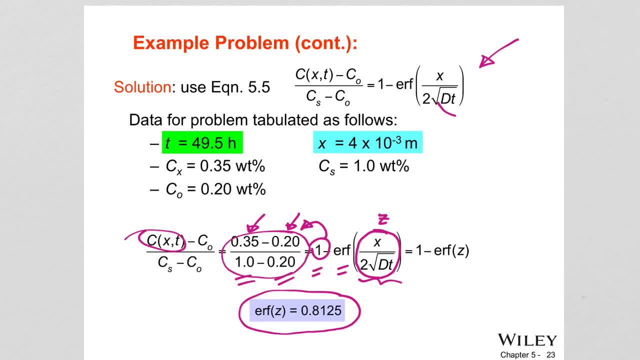 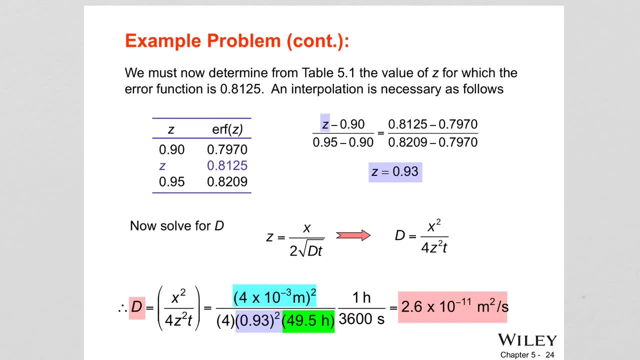 the term inside is simplified as Z, so you have to look at the tables for that, as I described to you guys. so these Gaussian error functions, they are tabulated in the tables you can find anywhere and it is also in our book, table 5.1 and. 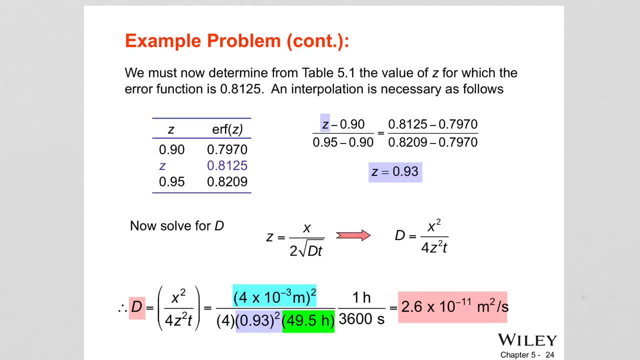 the part of a table, how we read the information can be seen in this, in this problem. so the part of the table is given, so we are given what in the table. we are given, if what is the error, function values and how we can, how it is. 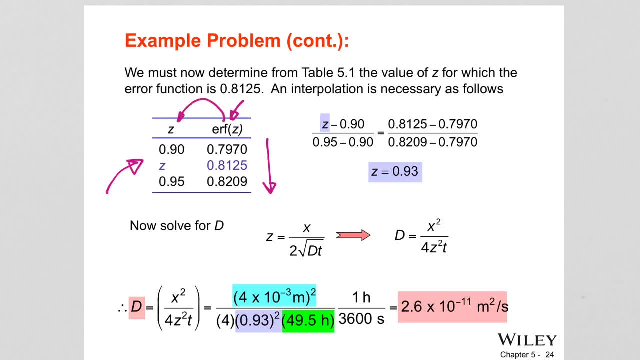 related to what is inside. so if the error function of Z is this, Z must be that okay. so we therefore we need to calculate it ourselves. sometimes the exact value of the error function might not be there in the table. that's one you need to do linear interpolation, and I hope you guys learned what linear interpolation is, and 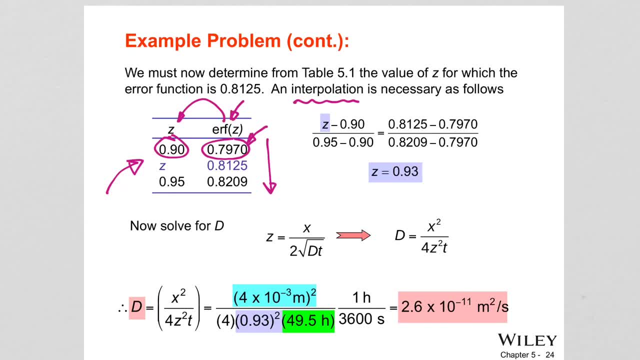 if you don't, i suggest you google it, and wikipedia is clearly explaining it, but we're gonna see an example here. okay, so we look at the table. we are seeing that error function is for this volume of error function inside the error function. is this right? and we also know from the 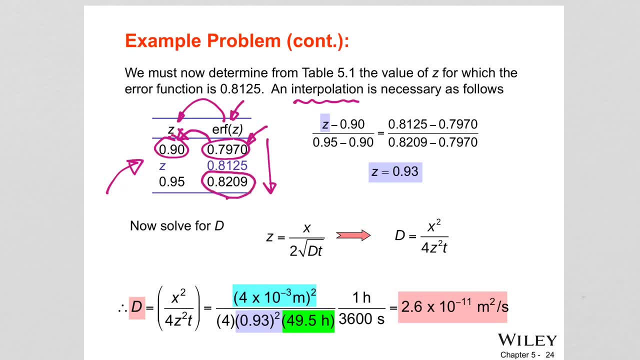 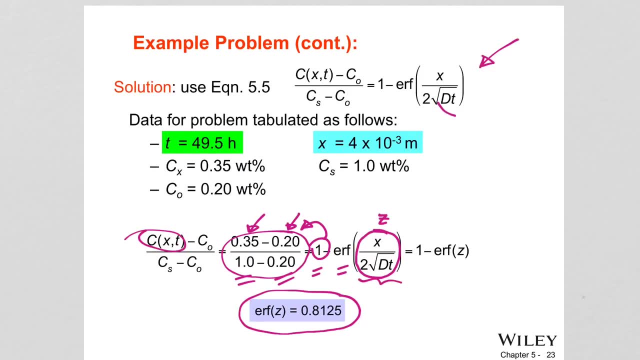 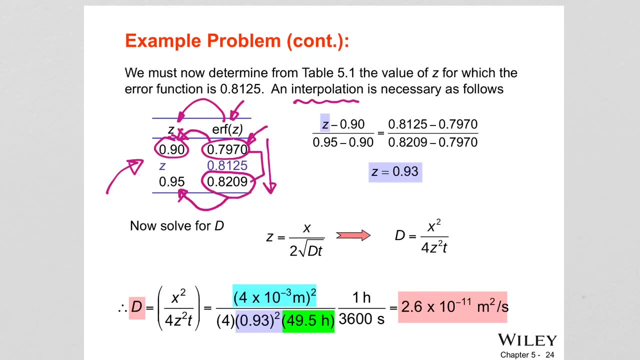 table. this is if error function is that our inside error function Z is 0.95. so now what is our volume for error function? our volume is 0.8125, so it is in between these. therefore, you put it in between, so I'm trying to find the. 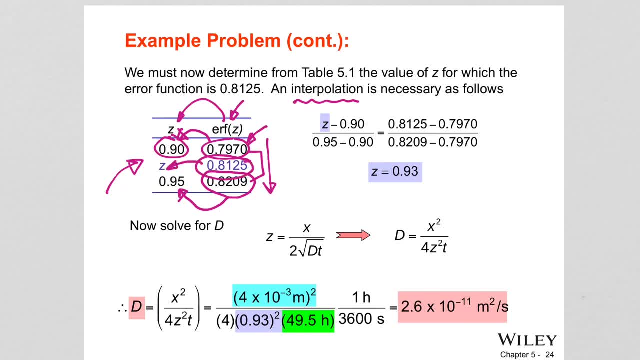 corresponding Z, and it should be in between 0.9 and 0.95. so to be able to do that with, we do something called linear interpolation. okay, let me erase all this now. okay, so this minus that over this. okay, so this minus that over this. 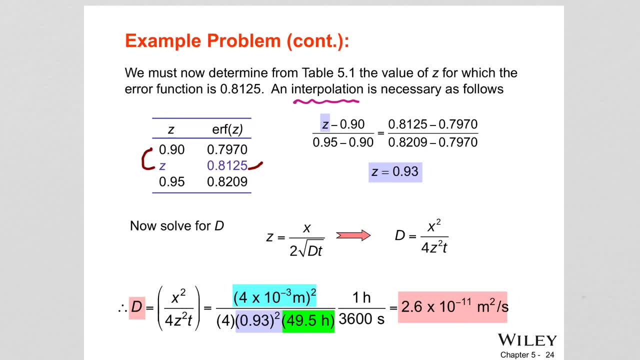 Let's say they do it differently. let me do it again, okay. So this minus that over this minus that is equal to this minus that over that minus that. So the linear interpolation actually comes from the fact that if you have a linear change in small ranges, like that, 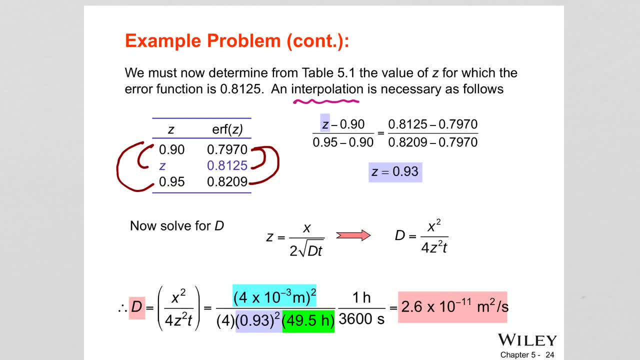 the change is always linear, approximated a linear change. and along the line, along the linear line, right along the linear line, the slope is the same. So if you take different points and calculate the slope for this curve, it has to be equal along the line, linear line. okay. 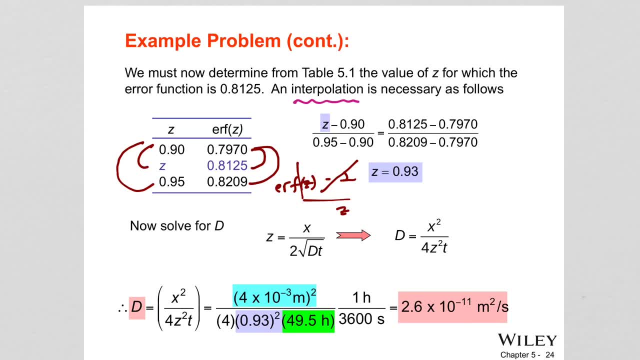 That's why it's called linear interpolation. So basically what we are doing is equilibrium. We are creating the slopes and trying to figure out an unknown value from here. okay, So I can also write it this way. So I can also say: z minus 0.9090 over 0.8125 minus 0.797 is equal to 0.95 minus 0.9.. 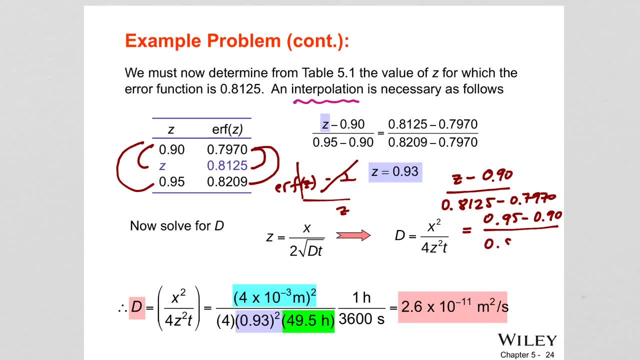 And it's equal to 0.8209 minus 0.797.. So there is also this way you can write it. It doesn't matter. At the end it gives you the same thing, okay. So it should give you the z. 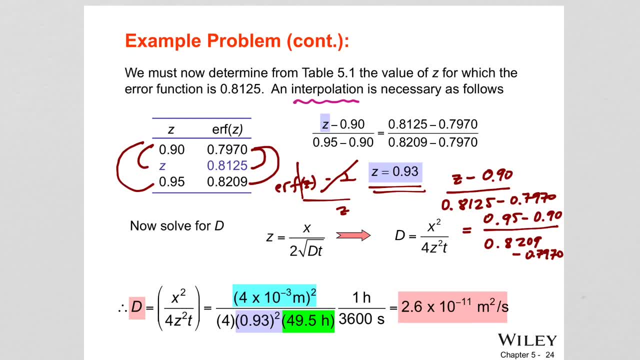 So we figured out inside the error function is equal to 0.93.. So this term here, this term is the value, It is 0.93.. Alright, so solve it for d. If you solve it for d, which I'm trying to figure out, it is x squared over 4z squared times t. 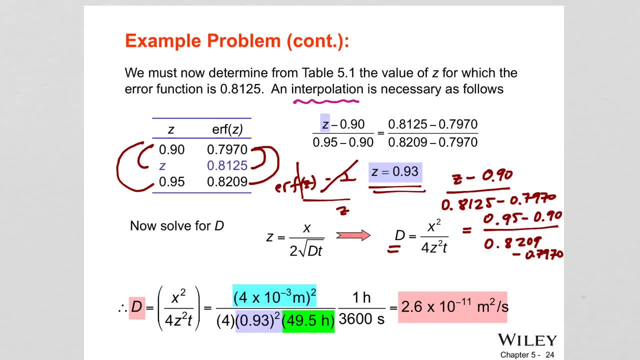 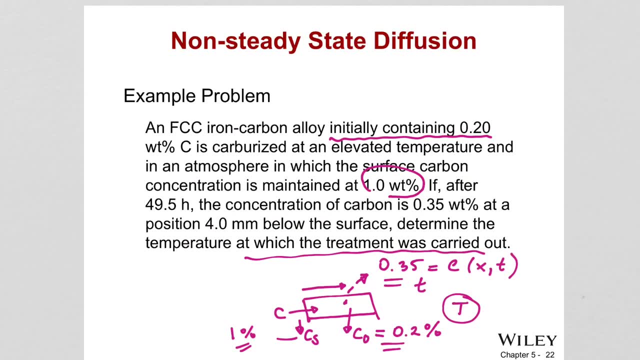 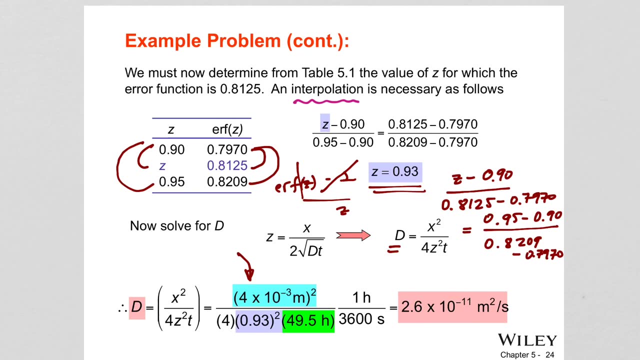 Okay, so all we have to do is now figure out the diffusion coefficient. And we are given the x. Yes, right, And of course, be careful with the units. okay, And we are, we calculated c. The time is given. 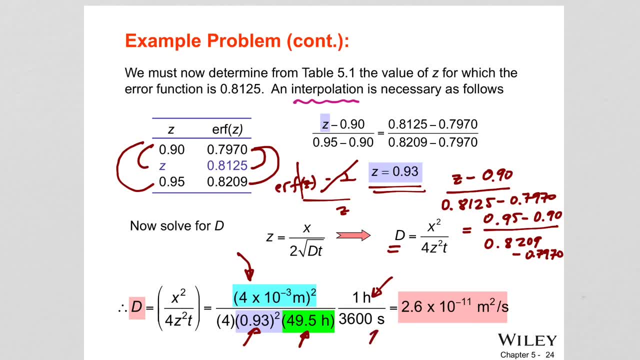 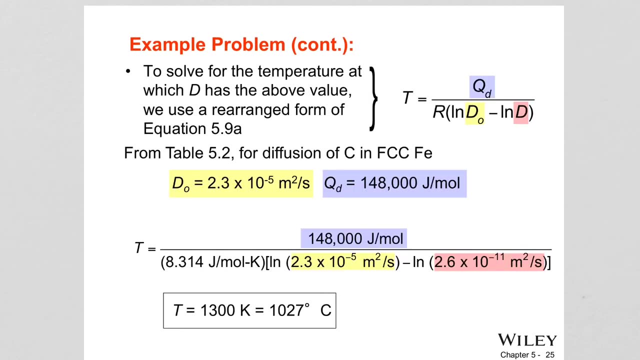 Be careful: Convert to seconds, Because the units of the diffusion coefficient is in seconds. So at the end you end up with calculating the diffusion coefficient. Now. next, remember, the problem is asking for the temperature And the diffusion coefficient is the dependence of temperature. 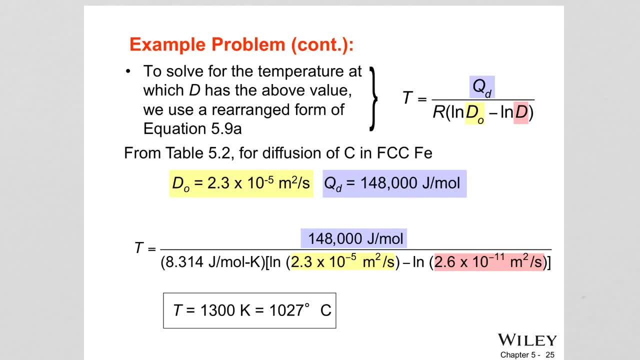 So I need to know the diffusion coefficient equation, which was: d is equal to d, naught exponential term minus q over rt. So if I know this one and if I know d, this one will be equal to c. So d is equal to d. 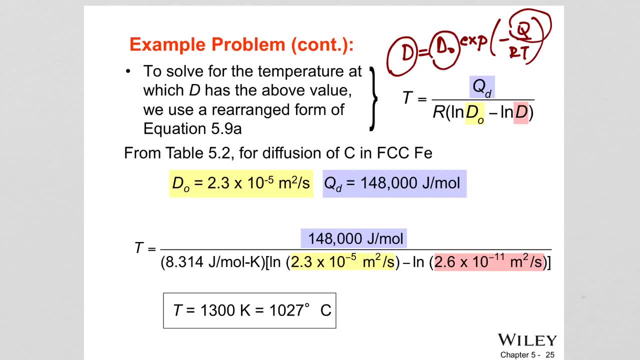 So d is equal to 0.. So d is equal to 0. So if I know this one, and if I know this one, and if I know this one will be equal to 0.. things for the that iron carbon system, then I should be able to, since this is a. 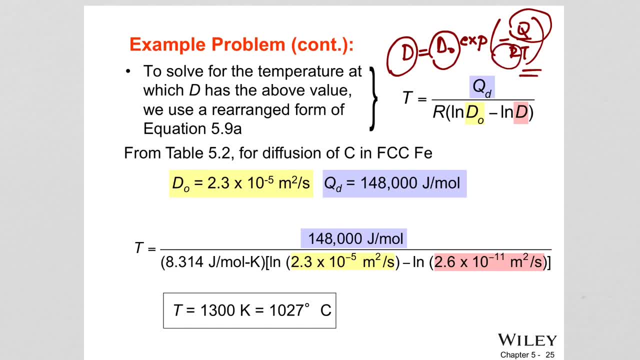 constant, I should be able to calculate the temperature. so in this case, this equation is sold for T and T is therefore activation energy over R. of course this is. they use the LN form. what was the LN form? L and D minus is equal to L and D, not minus Q over our T. okay, so solve this for T and it is going to. 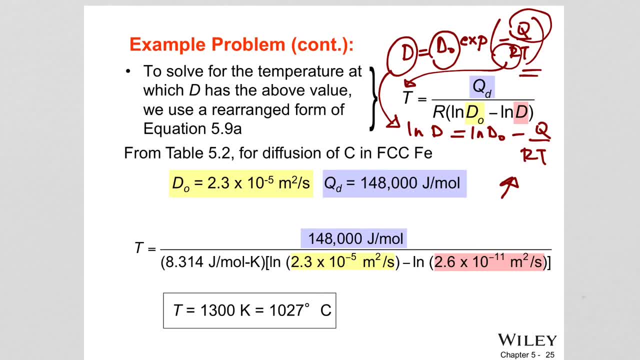 give you that right now, all you have to do. there will be certain tables where you figure out in the, in the talk in your book. it is the table 5 2. ok, Table 5 2 will give you information about the, not the, at the, not constant and activation energies for different. 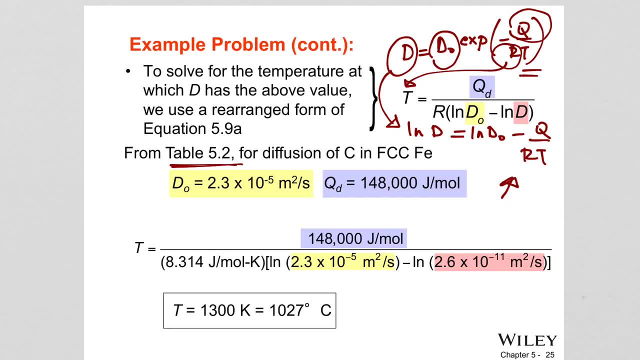 systems. so what do you have as a diffusing species? what is your host metal? based on that, you can read information about D- not this one- and activation energy. so try to look at the table to read this number, because in the exam I will give the table and you should be able to read these a. 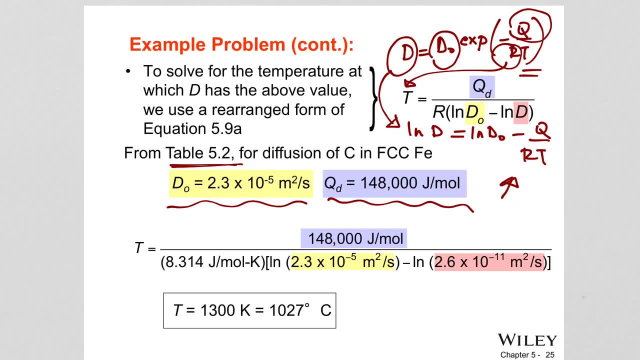 constants, depending on your system. okay, the systems are easy, very easily defined. be careful what your diffusing species here is carbon. what is the host medal? it is iron in FCC. okay, in FCC. okay, it is defined FCC iron. so, but he didn't have an explanation. there was nothing for an example from your. 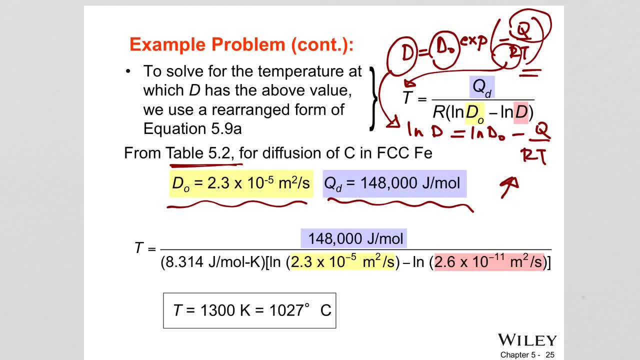 Based on that, you read the numbers of the constants d0 and the q. Okay, so look at the table and read these numbers yourself. okay, Don't just rely on the fact they are given in this problem, because in the exam or in your homework, basically you will have to read this table. 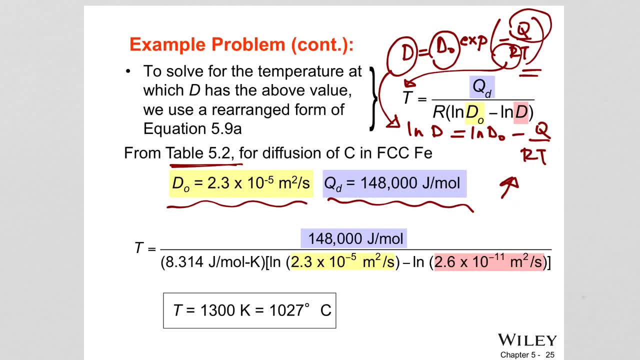 Okay, so from that information the temperature can be solved. basically, If you solve that equation, of course it's going to give you the kelvin in terms of kelvin. Depending on how it's asked, you can convert it to degrees C. but at the end this is how we find the temperature. 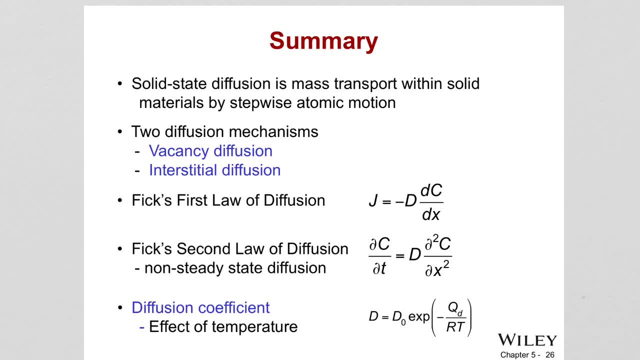 All right guys. so basically that's it in terms of this chapter. Okay, so we'll see you in the next chapter. We'll see you in the next chapter. Okay, so we learned diffusion, We learned the types of diffusions and we learned the diffusion mathematical equations, how they are calculated.